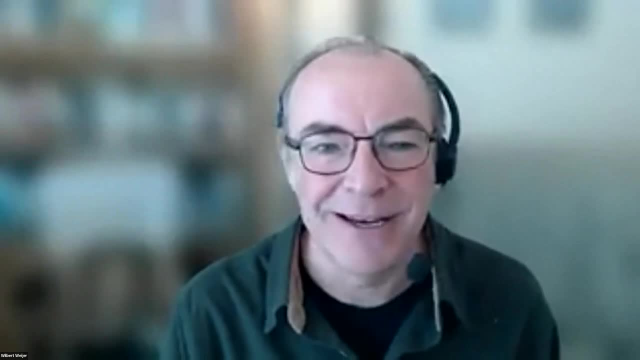 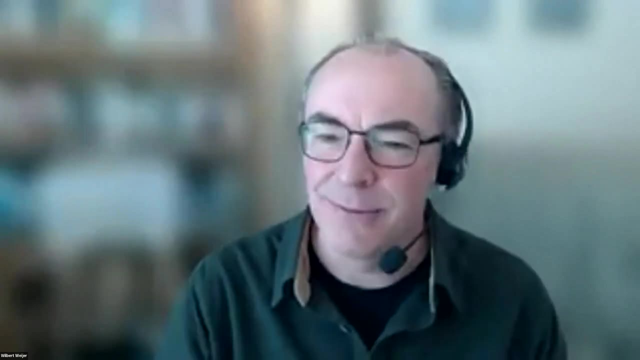 It's co-led by Dimitri and Zhu Jing, who are on the call as well, And it aims at connecting physical oceanographers, scientists and stakeholders that have a focus on the Arctic all across the interagency spectrum and also with international collaborators. 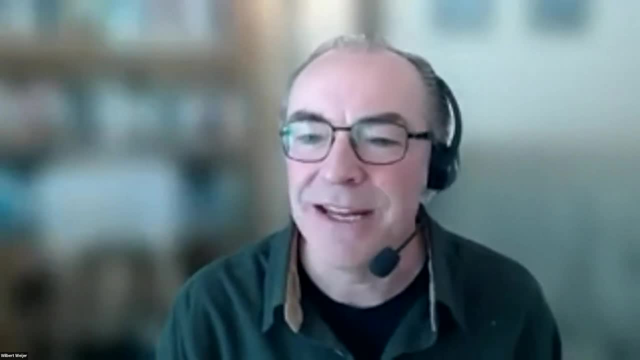 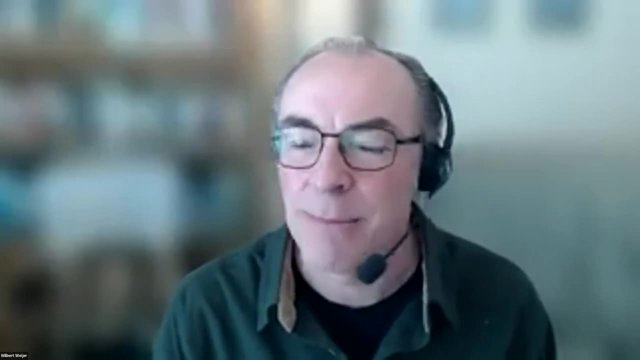 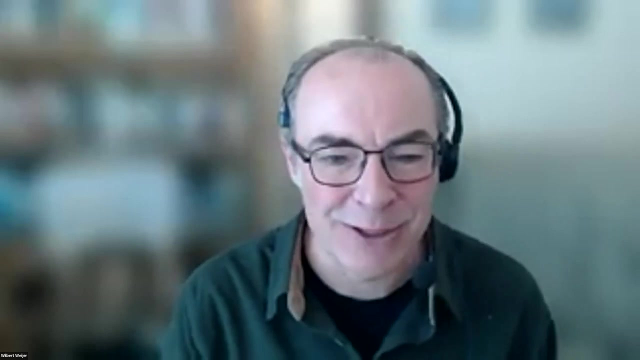 The modeling sub-team focuses on earth system integration and prediction through a hierarchy of modeling tools, And again it aims at connecting earth system modelers across the interagency landscape for enhanced collaboration and coordination of efforts, And this is co-led by Richard Colleter, who's on the call too, and by Reino Joseph as well. 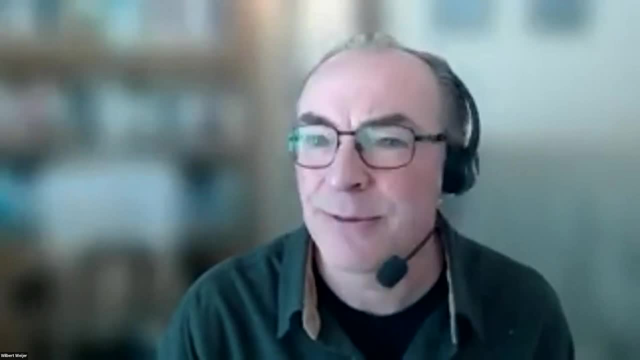 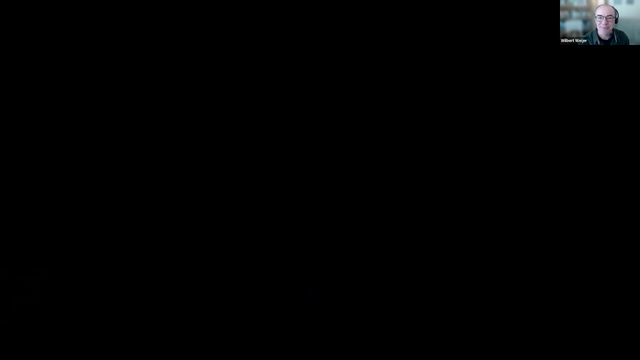 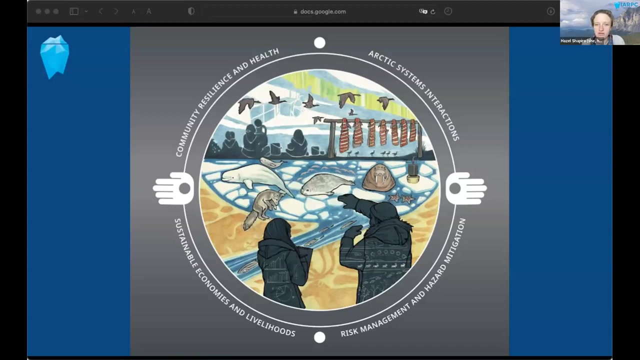 And I'd like to hand it over to Hazel For a couple of minutes to talk about the new Arctic research plan for 2022 to 2026.. Okay, Can you see those slides? Yes, we can Perfect. Thank you, Wilbert. Yeah, So just wanted to take a minute before we get started For those. 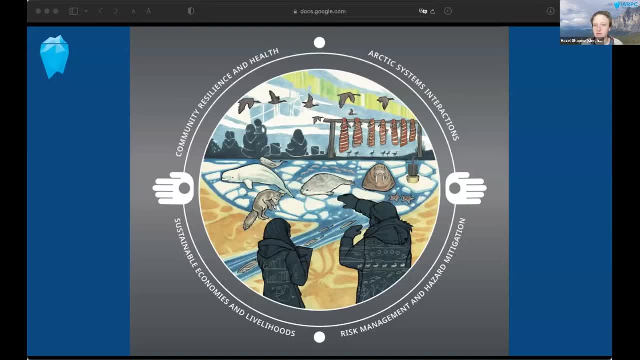 of you that are familiar with our IARPIC, this will be sort of a a familiar topic And for those of you that are new, welcome, and we welcome you to engage in this process as well. So IARPIC has been over the last maybe year plus. IARPIC has been working on 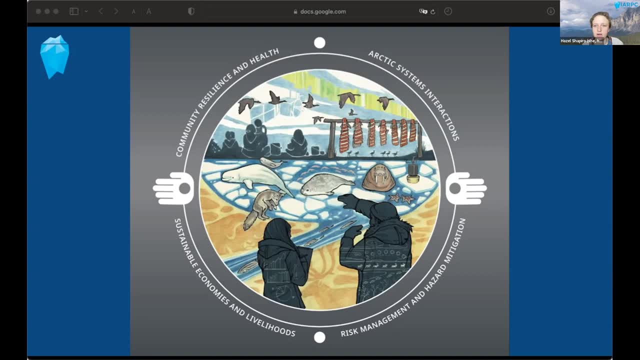 developing a new Arctic research plan. So we operate under five-year cycles of federal Arctic research plans And this new Arctic research plan provides a bold vision for federal agencies to nimbly and collaboratively help understand and support research, And I think it's a great idea. 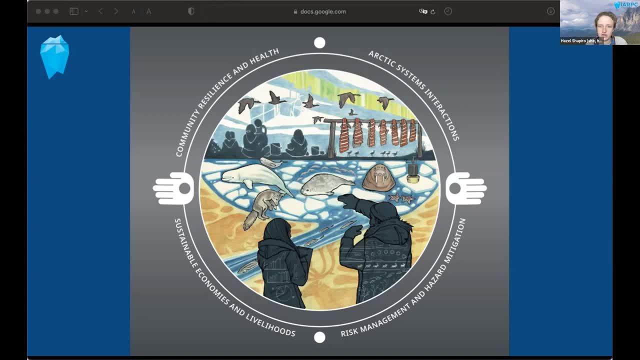 The Arctic is essentially a project built around goals and goals of the National Historic Authority, including national scientific and civil protection and human rights Strategies to include and support resilience in the face of the dramatic changes that are occurring in the Arctic, And so it is actually quite different than the previous plan, And this is a picture of the 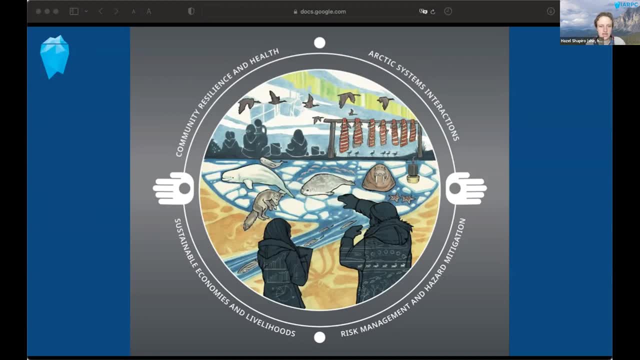 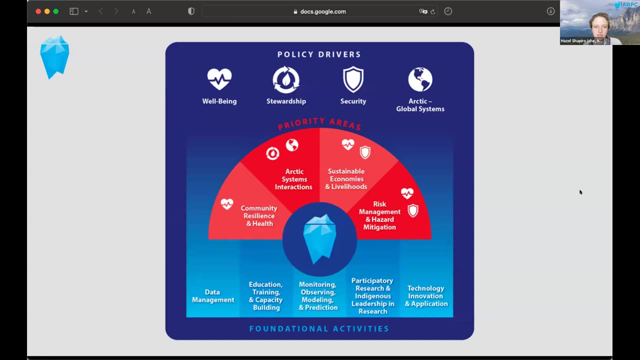 report cover, and it represents sort of the more holistic approach that this report is taking. thanks to artist Molly Treanor for the illustration and graphic designer Eric Klein for the overall layout. Okay, Thank you, Jill plan. if you took part in the plan development process, this will look familiar to you, though. 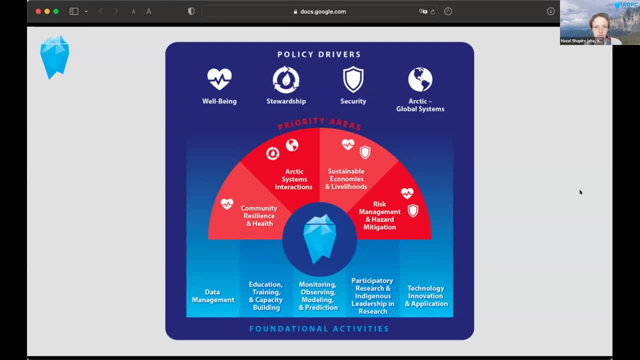 it has been updated since the plan was released in December. The top section shows the four policy drivers, and so you'll see that well-being, stewardship, security and Arctic to global systems, and that's where Arctic research directly supports US policy. And in the center you'll see: 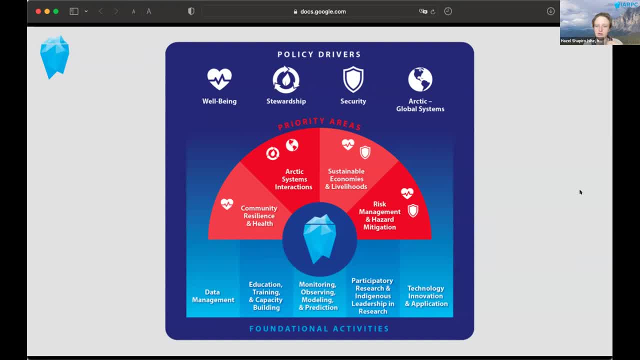 those four policy drivers too, are carried over from the last plan. And then what's new is that you'll see these four priority areas, which I'll go over in slightly more detail here, And I- yeah, I guess I won't read through that- And then, underlying that, there are five. 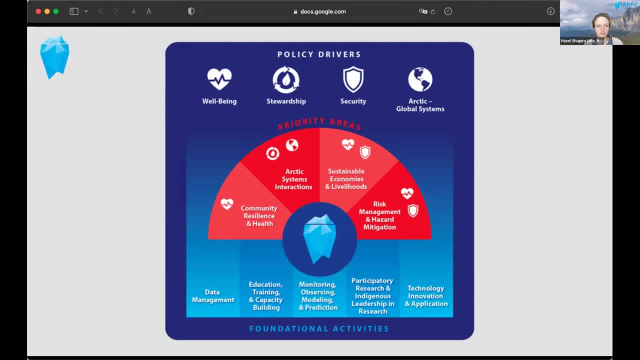 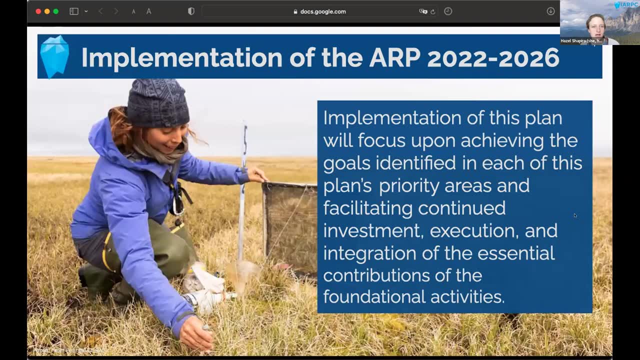 foundational activities that are supporting all of the four priority areas And um, as we recognize that the Arctic is changing at an unprecedented pace, and so, while this five-year planning cycle has allowed us to add in many emerging topics in the Arctic, we want to be 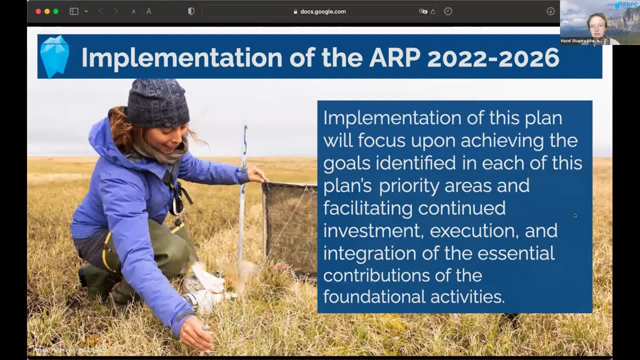 even more nimble than that. So we're working in this cycle of two-year implementation plans, And so right now, January through March, we're gathering ideas of what are the big topics that we really need to tackle within the next two years, And so 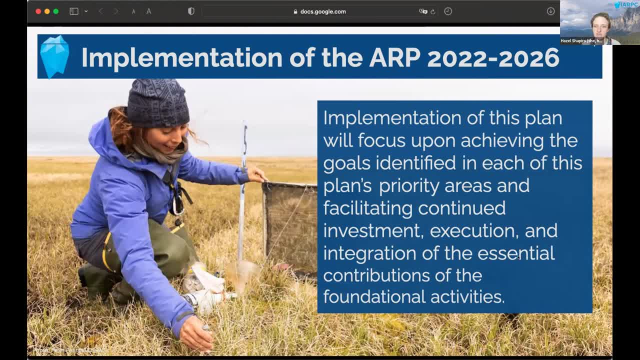 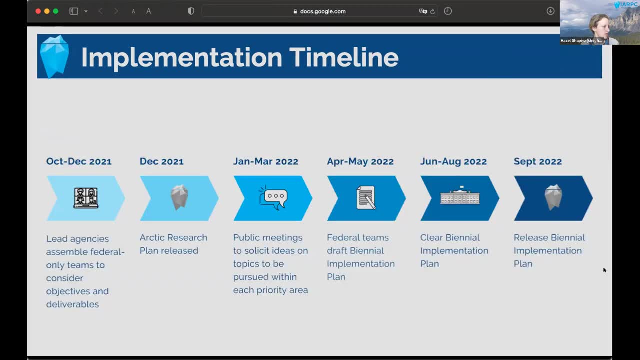 this, this presentation today, is really inviting you to share those ideas And maybe, Meredith, you could drop a link into the chat where folks can enter those ideas to be considered by the biennial implementation plan drafting teams. And so here you'll see the timeline And just to highlight again in this January to March phase, 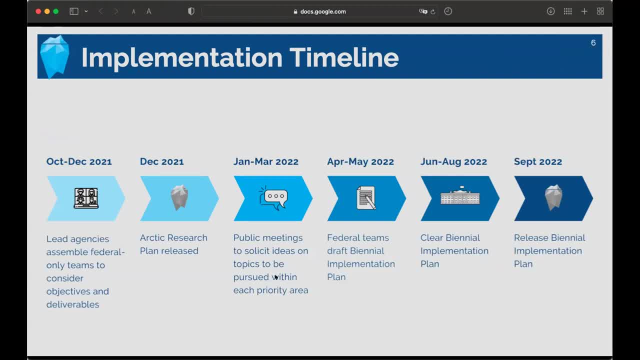 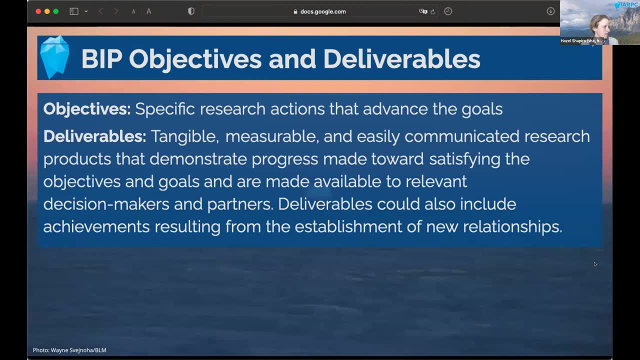 we are welcoming public input And then federal teams will write the biennial implementation plan and it will be released in September. I'm going to skip this side. It's just a differentiation between what an objective and a deliverable is. But if you have an idea, don't worry about that. Just let us know what you think is important. 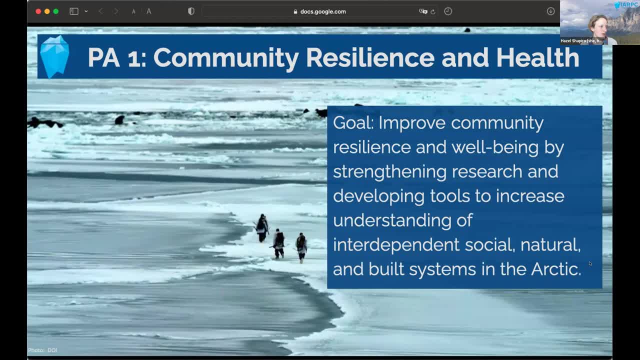 The four priority areas. I'll go through this really quickly, But the first one is community resilience and health, And we're aiming to improve community resilience and well-being by strengthening research and developing tools to increase understandings of interdependent social, natural and built systems in the Arctic. 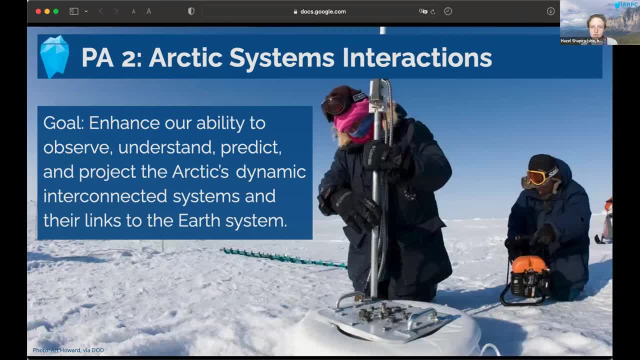 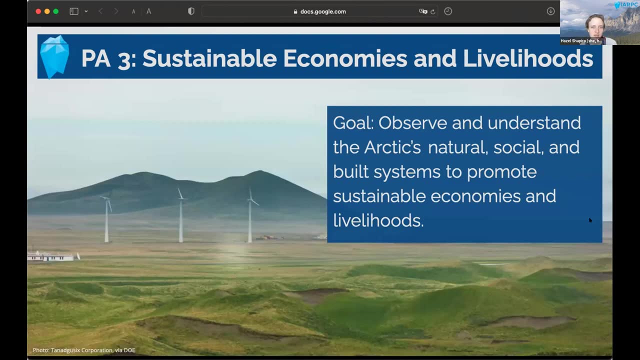 The second one is priority area two, which, if you've been involved with IARPIC, many of the sort of natural science activities will fall into this priority area two: Arctic system interactions bucket. Priority area three is sustainable economies and livelihood, And we'll be aiming to observe and understand the Arctic's natural, social and built systems to promote sustainable economies and livelihoods. 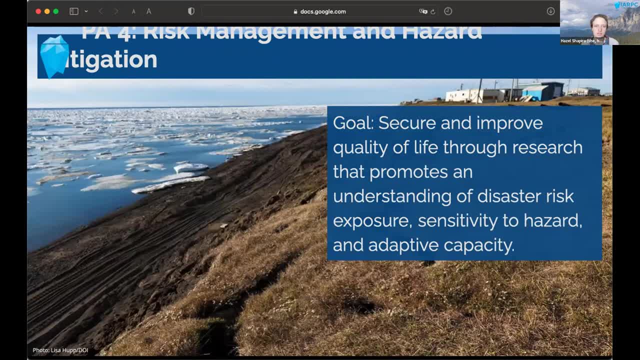 And then, just very briefly, four is focused on risk management and hazard mitigation, And so, if you have an idea to suggest, making a clear tie to one of these four priority areas is really the best way to get your idea into the implementation plan. 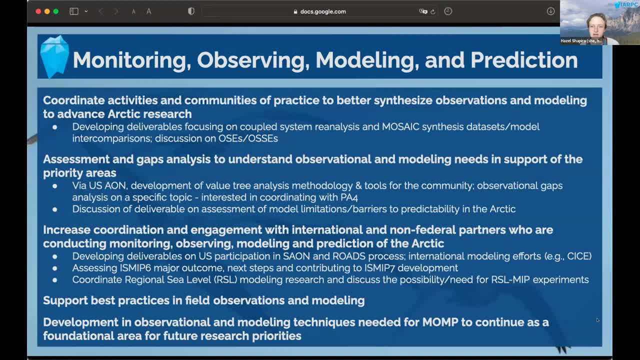 Oh, it looks like I skipped the slide, unintentionally, with the five foundational activities outlined, But you can refer to the website for that information And I just did want to highlight that this one is probably most relevant, especially to the modeling folks on this call. 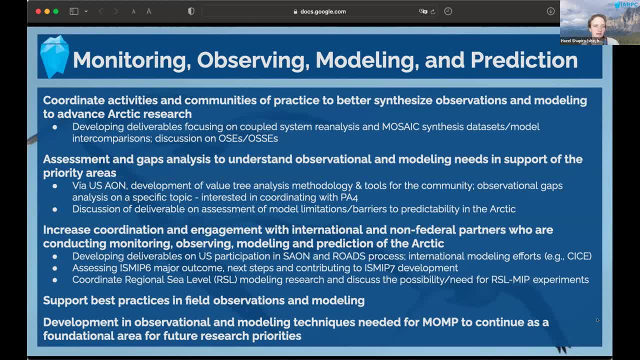 So this monitoring, observing, modeling and prediction foundational activity, And there's a couple of directions that the drafting team is considering for that, And so if you have input there, please let us know, Meredith, anything that I missed Or anything else that any questions that people have. 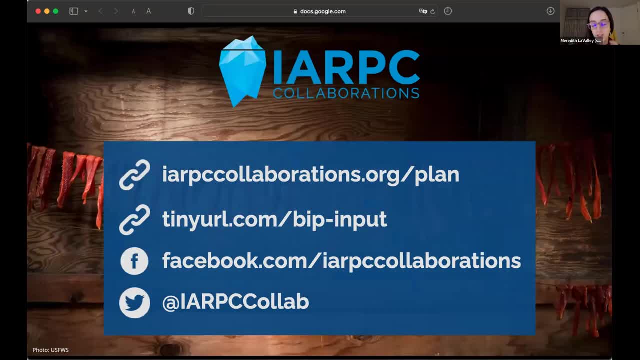 I will just add that I'm dropping one more link into the chat, And that is an informational session we're holding on February 15th, where there will be more detail about this: the Arctic Research Plan and the biennial implementation process. Great thanks. 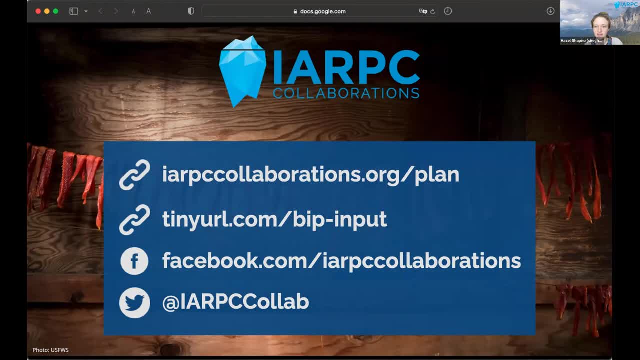 I recognize that was really quick, Especially if you haven't But involved in the plan process. But please do put questions in the chat Or I can drop my email in there And if you have more questions let me know. And with that I'll pass it back to Wilbert. 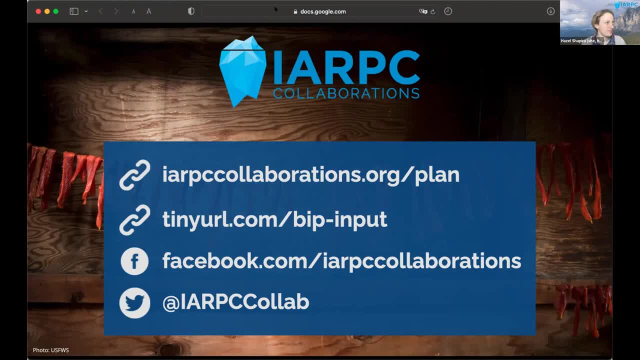 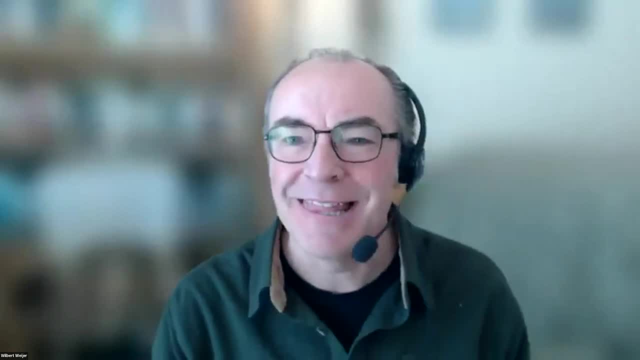 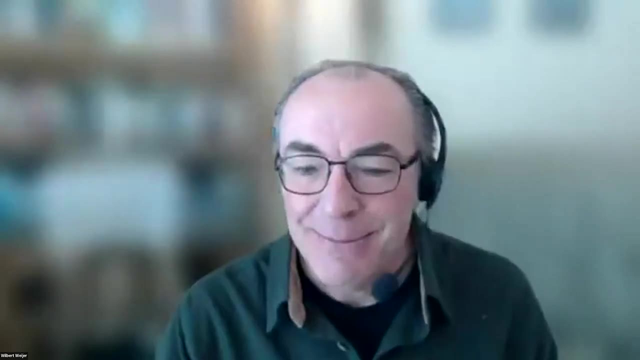 And I know we have a full agenda today. Thanks very much, Hazel. This was very useful, I think, to give people an overview of what is going on in IARP land. So today we'll be talking about oil spill response and remediation. 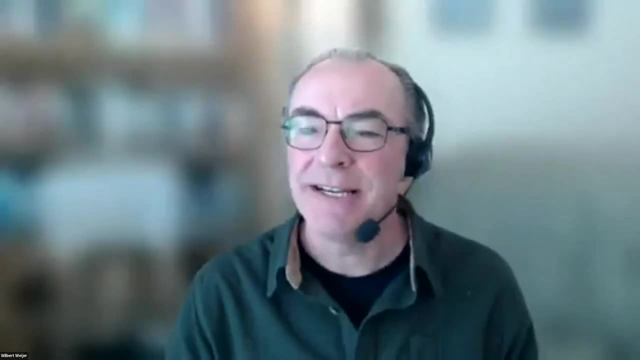 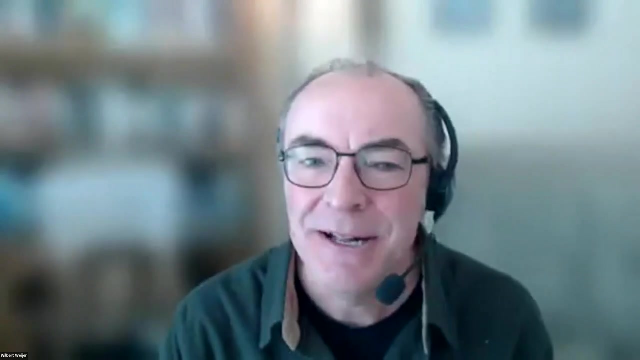 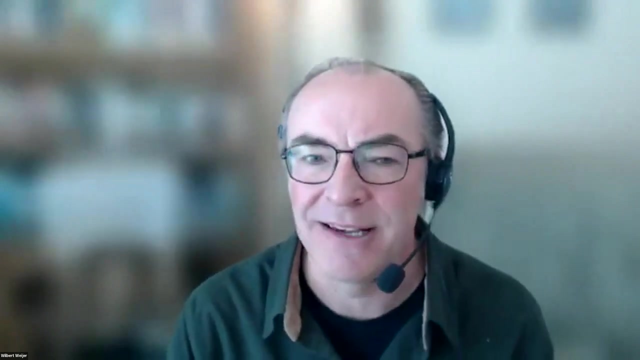 It's obviously a challenging task everywhere, but no more so than in the Arctic. Modeling plays a critical role in predicting the pathways and dispersion of oil spills, And in this webinar we will hear from two teams that develop and apply capability in the area of oil spill modeling in the Arctic. 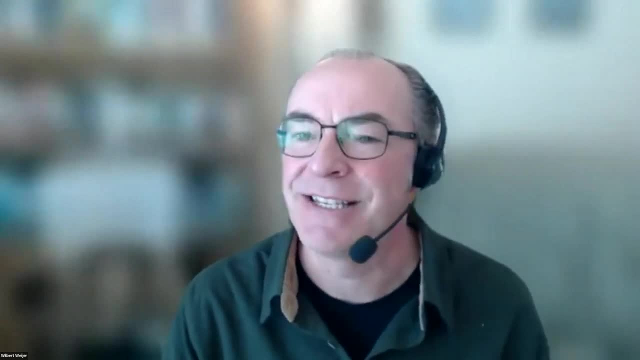 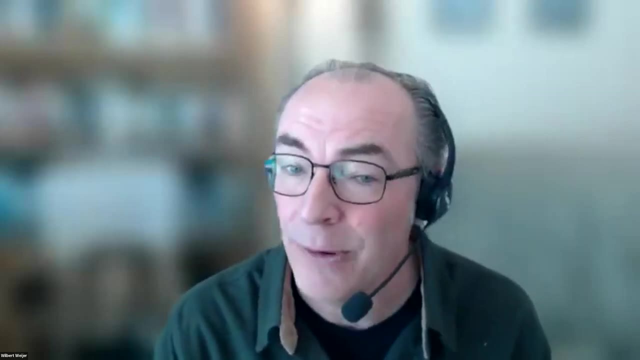 And hopefully we'll have some time to discuss the role of interagency and international coordination and collaboration on that as well. I think this team is relevant to priority area number four, That is, the oil spill model That Hazel just presented on risk management and hazard mitigation. 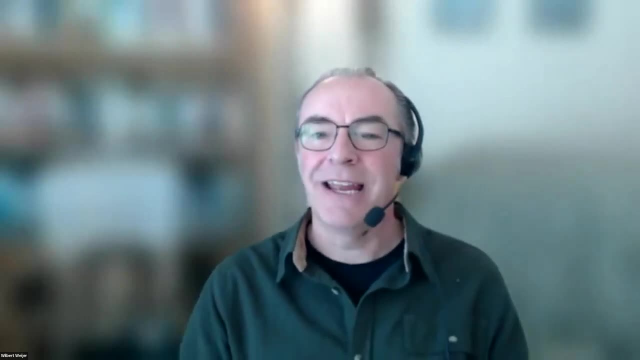 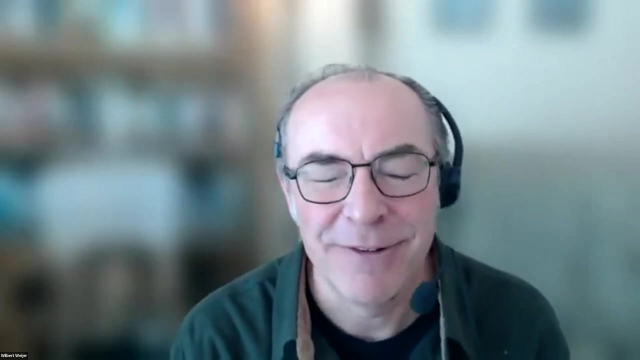 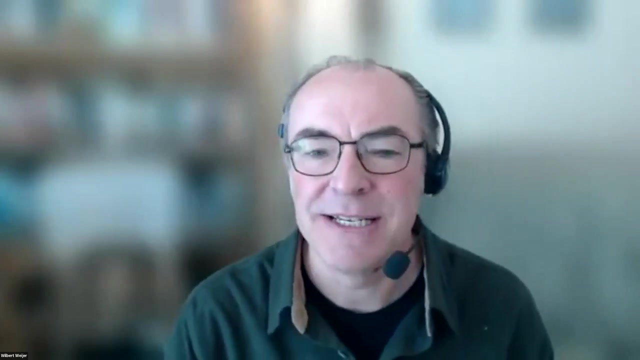 So we'll start with the presentation by Amy McFadden. She is an oceanographer in the OR and ARS oil spill response program at NOAA. She's got a PhD in physical oceanography from the University of Washington And she participated in the international collaboration in response to the Japan tsunami marine debris event. 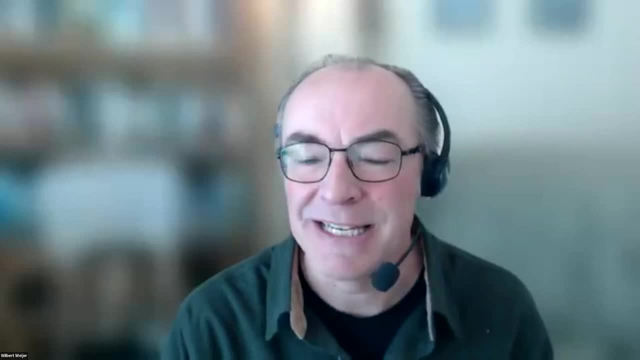 And she's currently project manager at the IARP. And she's currently project manager at the IARP. And she's currently project manager at the IARP. And she's currently project manager for the GNOME oil spill modeling suite. So with that I hand it over to Amy. 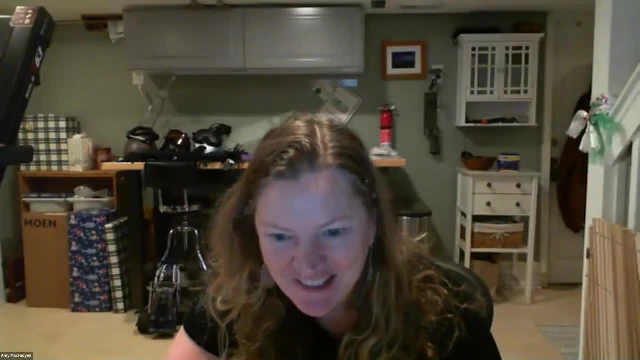 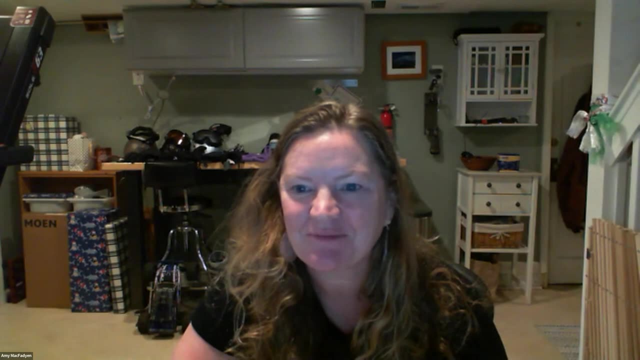 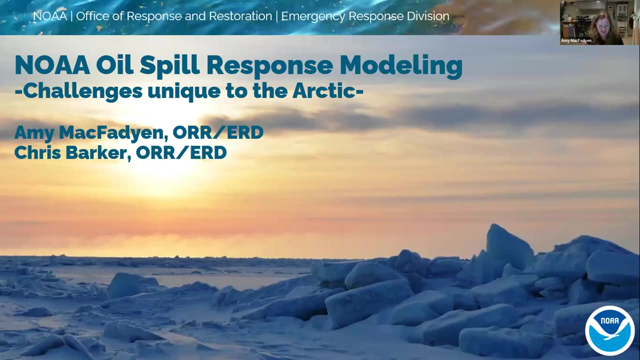 Thank you very much for the introduction. I'm going to try to share my screen now. Hopefully I can make this work properly, Okay, So if that worked well, you're looking at a lovely picture of Arctic Sea. Let me just get my slides up in front of me so I can see. 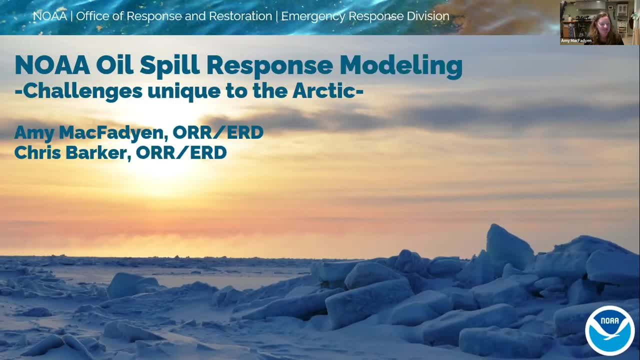 Yeah, this picture. So my research has never really been focused specifically on the Arctic. It was, you know, physical oceanography of the Pacific Northwest coastal zone initially, And then more recently with NOAA oil spill response modeling, both as a practitioner of using models for response as well as developing models. 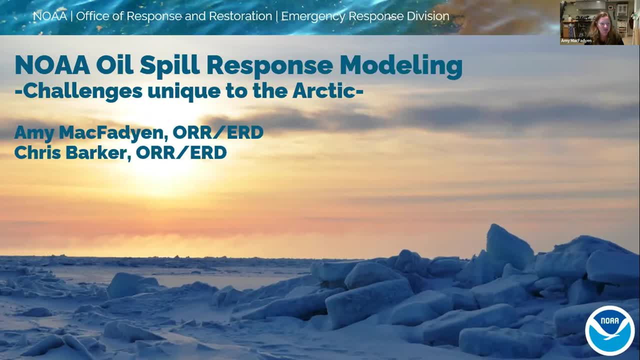 But I did have the good fortune to travel some years ago To Barrow, Alaska and Wainwright in a workshop that was focused on trying to incorporate traditional ecological knowledge into response planning And it was just an absolutely fascinating experience. I got to hear, you know, really engage with some of the local indigenous people and learn some of their. 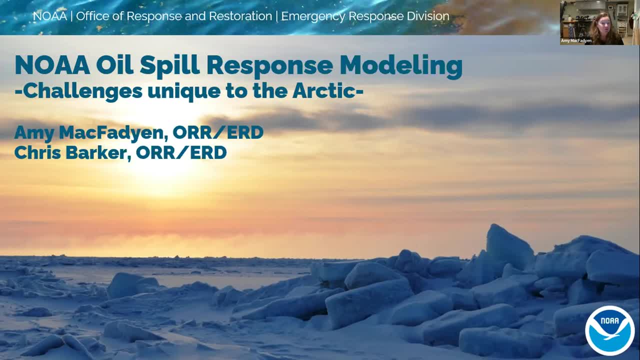 you know some of their experiences and concerns about oil spill response, specifically in the Arctic, And so I just thought I would share that as a start, as we're looking at this wonderful picture Of the ice edge off of Barrow, the land-fast ice. 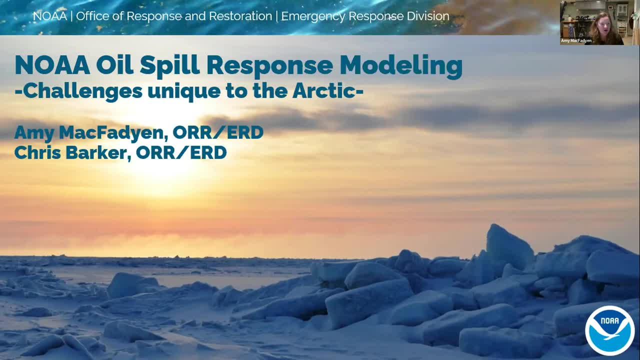 I just want to acknowledge my colleague, Chris Barker, who's also on the call. Chris and I pretty much together, lead the Nome development. You know so detailed algorithmic questions I will probably defer to Chris, But I'm going to hope to hopefully give a general overview of our oil spill response modeling program. 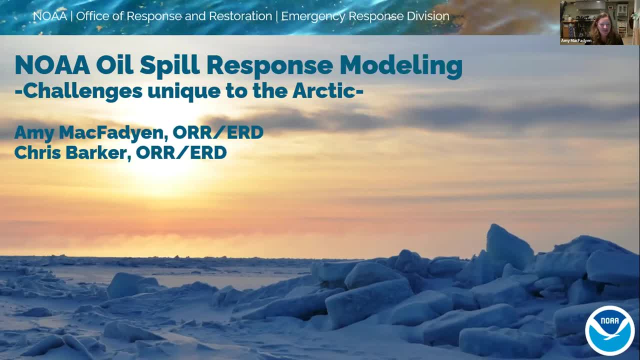 And then try to highlight some challenges Unique to the Arctic. I'm not going to get too into detail on the specific oil and ice modeling interactions Because I think Tora is going to cover that after my talk. So this will be more general about oil spill modeling and response. 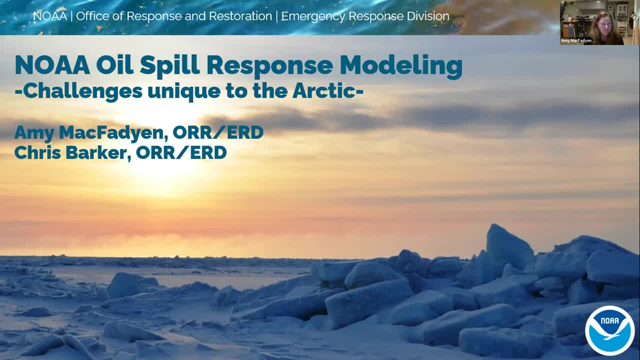 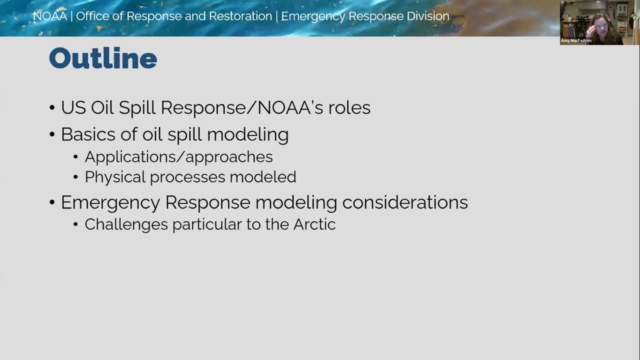 Specifically focused on response modeling. I do have just a brief outline of what I'm going to go over. I thought I would start with just a really quick overview of the kind of US You know within the Arctic, Within the United States. 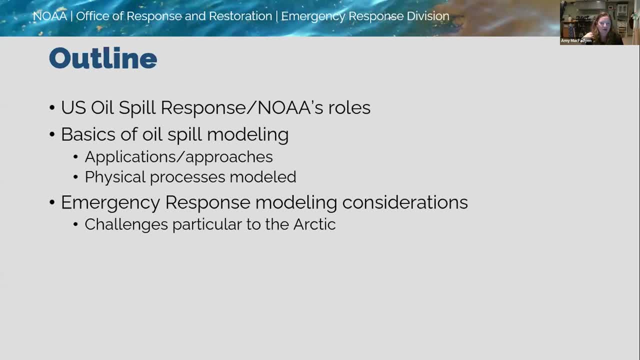 The oil spill response framework that we work under, Just to kind of show how NOAA and my office fit into that framework. And then, as I said, some basics of oil spill modeling, Different applications for oil spill models and approaches that we might take for those applications. 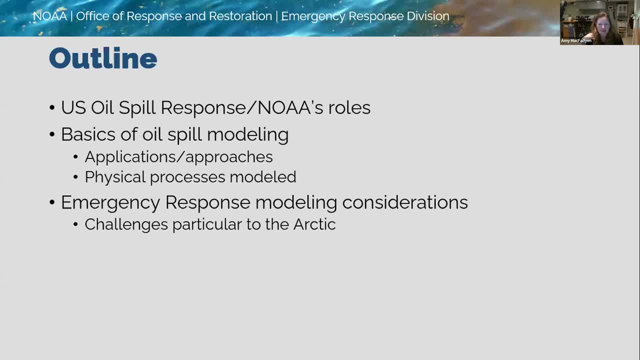 And I will go over briefly the physical processes that are typically modeled in oil spill models in general And then, as I said, more specifically to response modeling considerations And challenges, particular to the Arctic. So yeah, as I said, I was going to start with just a very brief overview. 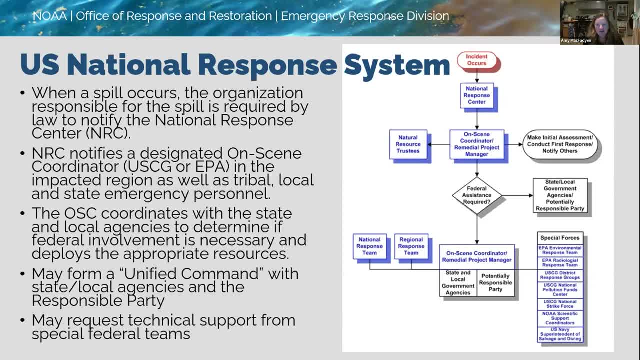 This is my most boring slide And I'm sorry I'm not going to spend too long on it, But I think it is, you know, informative to think about the framework that we work under. So within the United States, we have the National Oil and Hazardous Substances Pollution Contingency Plan. 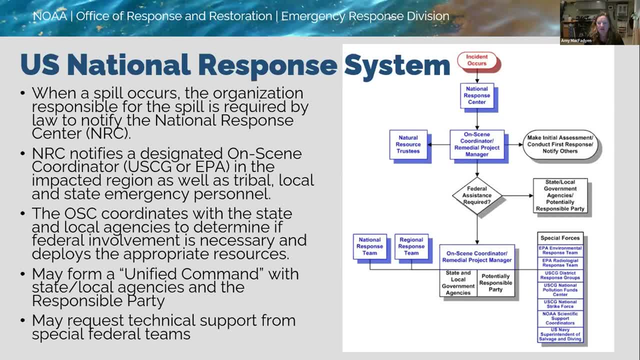 Which we call the NCP For short, because that's way too much of a mouthful. So the National Contingency Plan basically establishes this national response system, Which is the federal government's response management system For emergency response to releases of hazardous substances into the environment. 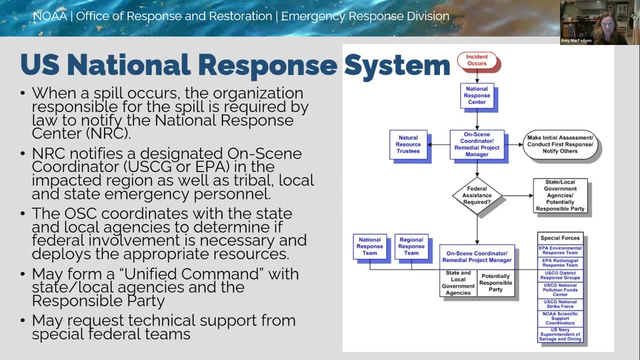 So this includes discharges of oil into coastal waters. Basically, when a spill occurs, the organization responsible for the spill is required by law to notify the National Response Center. They in turn notify a designated online response center. They in turn notify a designated online response center. 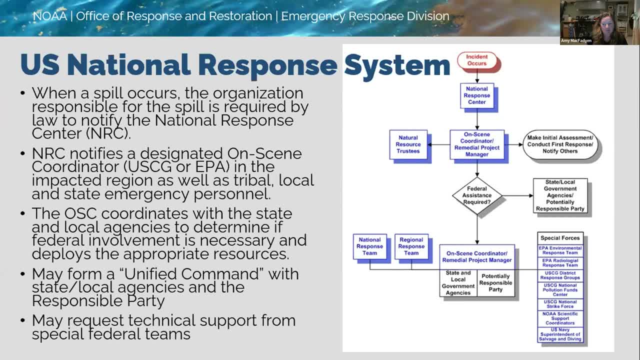 They in turn notify a designated on-scene coordinator. These are federal officials pre-designated by either the EPA or the US Coast Guard. In the case of spills in marine or navigable waterways, it's generally the US Coast Guard. 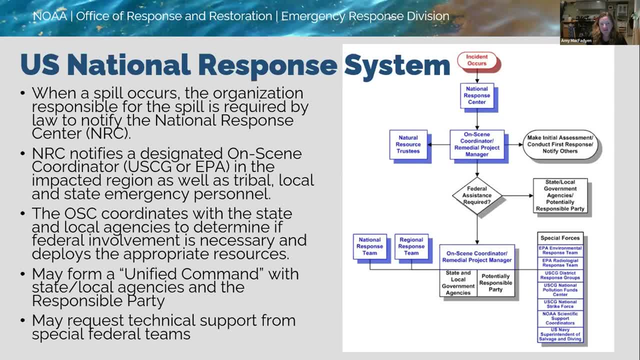 So the on-scene coordinator then coordinates with the state and local agencies to determine if federal involvement is necessary And then deploys the appropriate resources If the spill warrants it. they'll form a unified command with state and local agencies And then the responsible party. 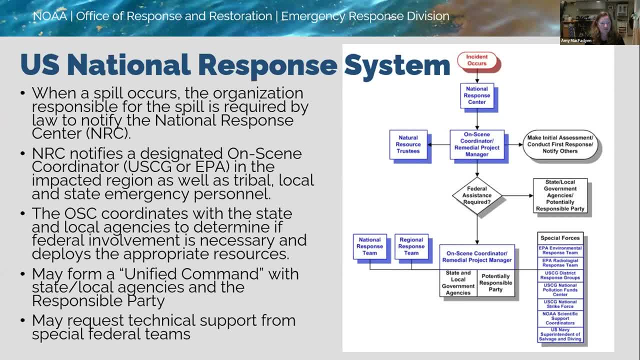 The spiller of the oil in this case is also invited to be a part of that unified command So they can really be working together to respond to the oil spill to try to mitigate the damage. So this is finally where NOAA comes in. So the unified command can request technical support from these special federal teams that are this list on the lower right side of this flowchart. 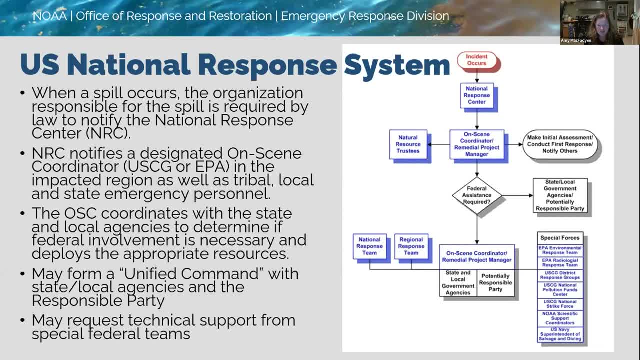 So the different special forces teams that are called out in the National Contingency Planner. So the special forces teams that are called out in the National Contingency Planner there, including down the second one from the bottom, NOAA scientific support coordinators. So our office, the Office of Response and Restoration within NOAA, in our emergency. 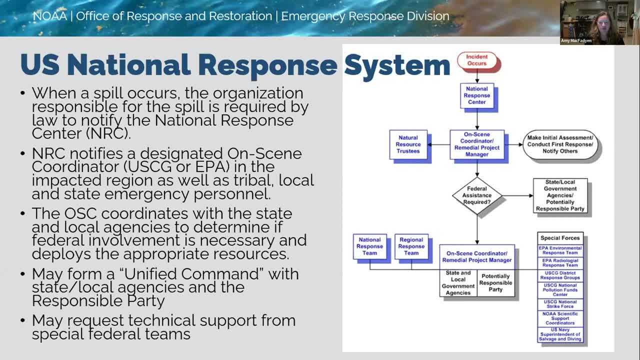 response division we have a group of scientific support coordinators who are regionally based and if a spill occurs in their, in their area, they then are that input to the, to the on-scene coordinator, and they reach back basically to us in Seattle for for information on whatever the 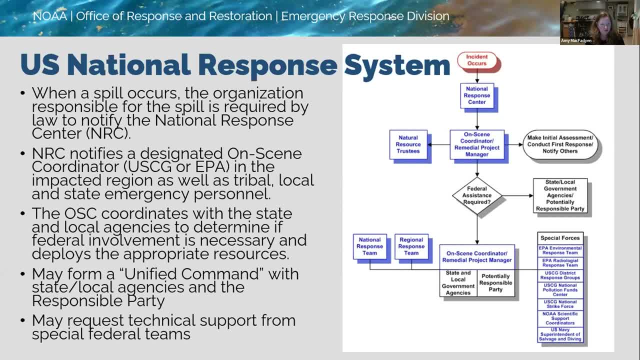 questions at hand may be The other part of this flowchart. on the left, it just calls out the national response team and the regional response teams. These are representatives from various federal agencies that have expertise in various aspects of preparedness and response. They're 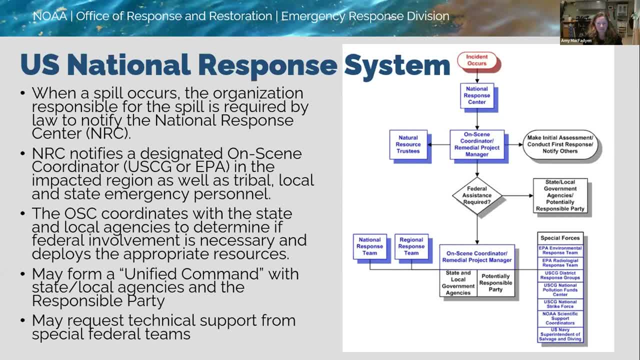 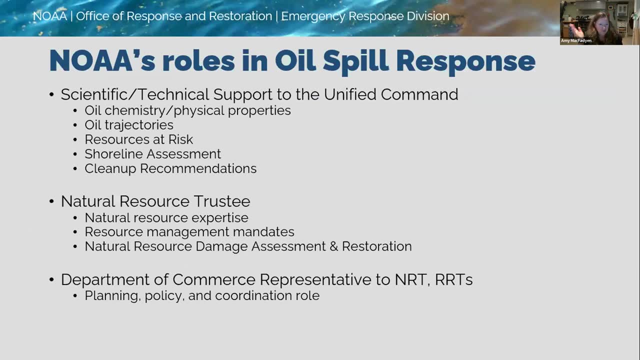 typically more involved in in planning and policy guidance prior to a spill. but they can provide support for that To the, to the unified command, if asked. So drilling down from there to NOAA's various roles in oil spill response. So, as shown in those kind of special teams in direct input to the unified command in the 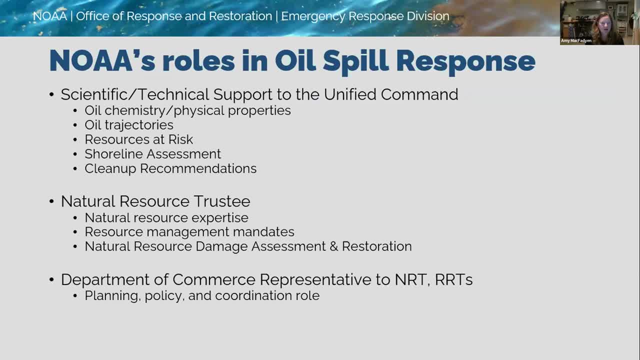 areas of scientific and technical support. So that might be questions about the physical properties of the oil, its chemistry, its toxicity. where is the oil going to go? what resources are in the area, shoreline assessment techniques for for serving the oil and making recommendations on on cleanup. 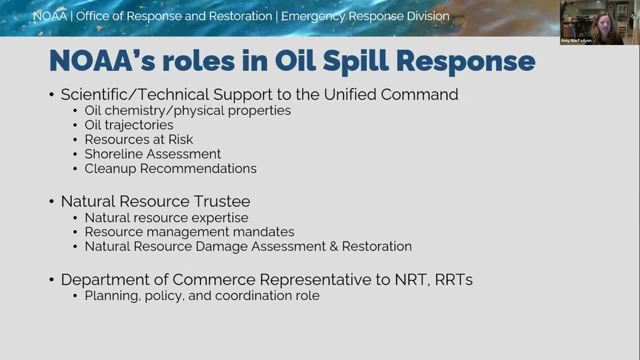 So that's the one one big role that our office plays in oil spill response And then under various laws such as the Oil Pollution Act, Clean Water Act, CERCLA and others. NOAA is also identified as a natural resource trustee for the public's natural resources. 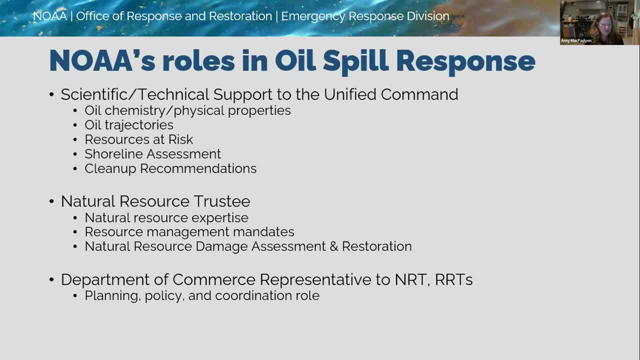 So there's rules associated with that national trustee role, and that includes, in the aftermath of a spill, the natural resource standard. And then there's the damage assessment and restoration, So determining the impact of the spill, actually putting a monetary value on the damage, and 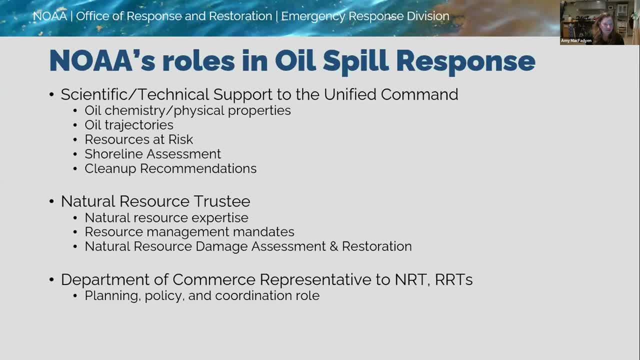 using that money towards restoration projects. And then the final rule I've called out, there is NOAA is the Department of Commerce representative to those national response team and regional response teams. So that has that has a you know before a spill- the planning policy and coordination rule. 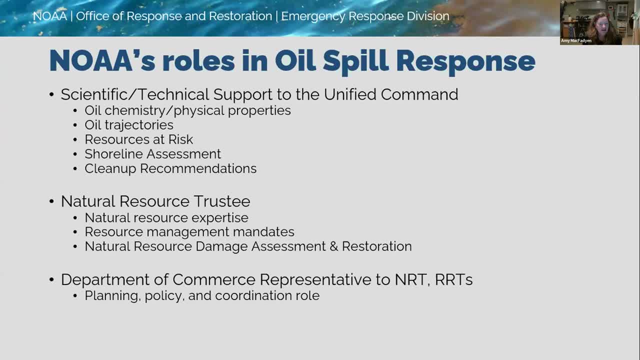 And then there's the oil spill modeling, now as promised, but this kind of illustrates three different areas where we might use oil spill modeling to support oil spill response. So during a spill, in that scientific, technical support role, you know, doing emergency response trajectories for example, and then in the national resource trustee role, modeling can be used to help. 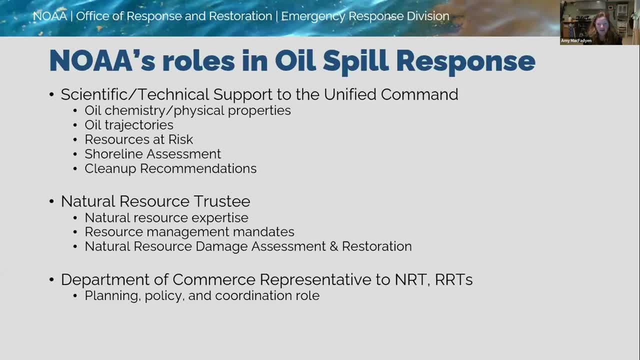 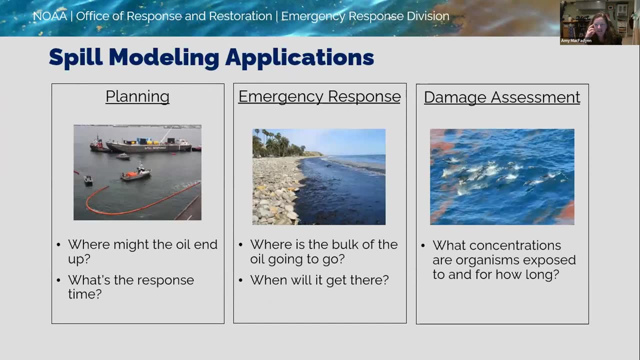 look at the damage assessment, The impact of a spill in the aftermath of a spill. So hindcast modeling and then planning and finally planning and preparedness activities. also, modeling can provide support for that as well. So these three different applications, I've kind of spelled them out in more detail here. 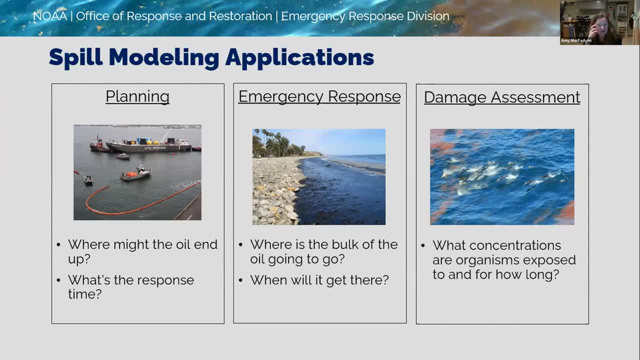 to make the point that these different applications- planning, emergency response, damage assessment- require different modeling approaches, as they're generally asking very different questions and have very different constraints in terms of the timeline in which information is needed and the information available to input into an oil spill model. 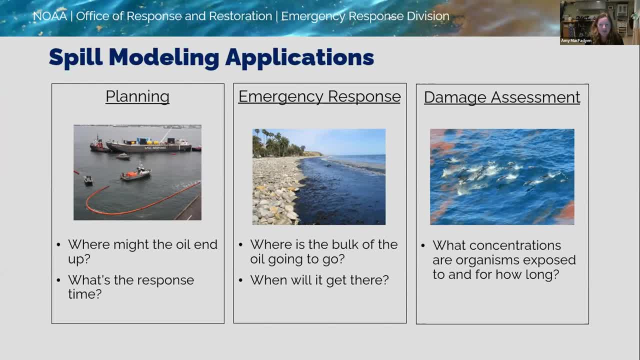 So for planning and drills, we're trying to run um uh models to capture what, what might be most likely to happen or or, if not most likely, what is the worst that can happen. Um, you know, you might want to answer both of those questions, because there may be. 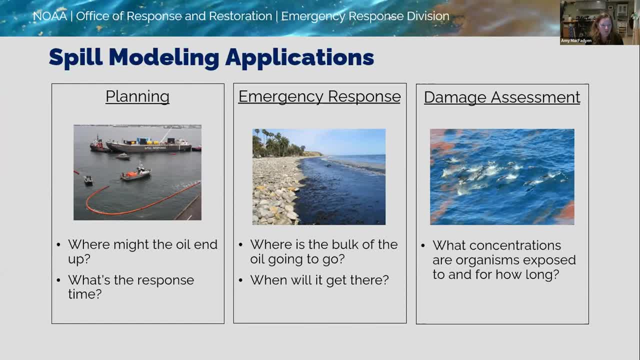 particular sensitive resources in an area that you're most concerned about. so you want to know what, what is the probability of impacting those resources. So we're asking questions like: where might the oils end up given a spill from a certain location, and how much time do we have to respond so you can develop response plans? 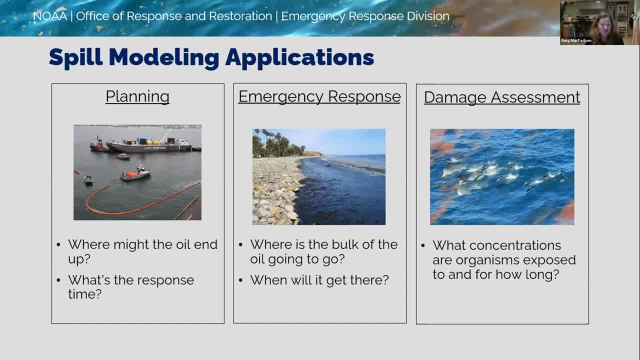 Then emergency response. Here you know, we're trying to figure out what's going to happen now or tomorrow so we can immediately take action and try to mitigate damage to a spill. So where is the bulk of the oil going to go and when will it get? there are kind of the key questions. 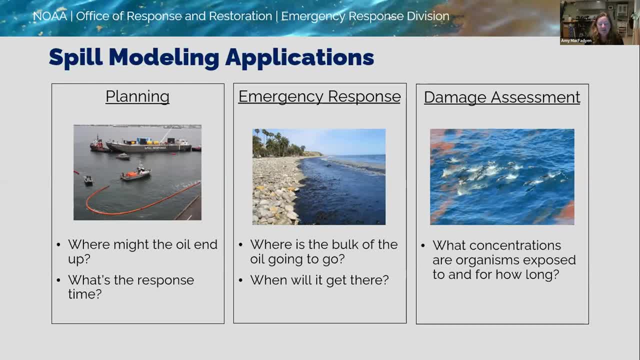 And then damage assessment, So that's in the aftermath of a spill. you know a more perhaps holistic modeling approach where you're really trying to get at concentrations that organisms are exposed to and the duration of exposure. So potentially a much more sophisticated or complicated modeling approach might be needed there. 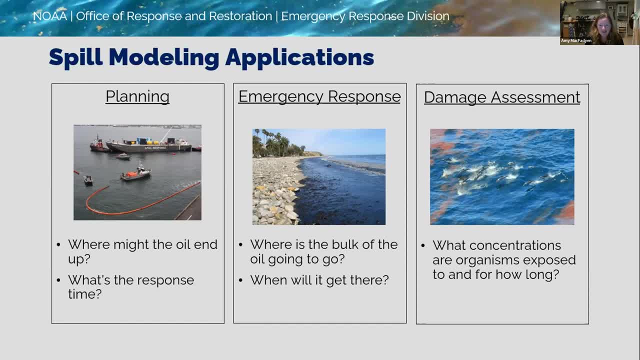 Whereas emergency response, we generally have very limited information going in and it's it's kind of a two way street of the, the timeliest answer. we, you know the best answer we can give in the short time frame to to inform the response. so the, the model, the underlying model, regardless of the approach, 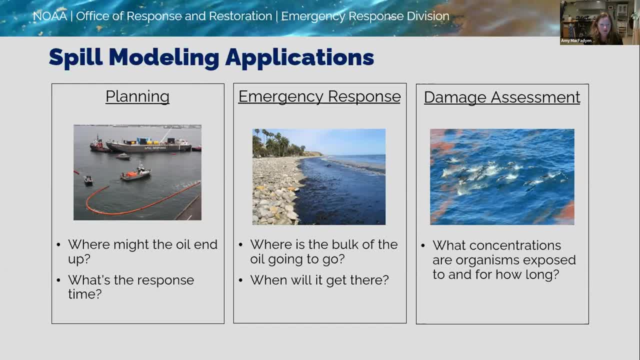 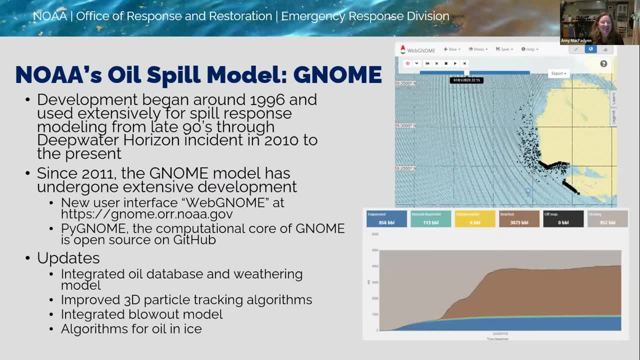 the underlying model that we use um is the same. it's a model that we develop um in-house, which we call gnome. the general noah operational modeling environment is what that acronym stands for, so this is a model that's been developed at noah um long before i began in in about 2009. 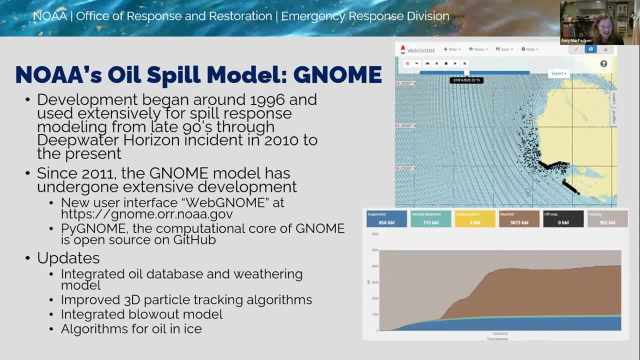 so it started in 1996. um was the first iteration of gnome and it's been used extensively for spill response since then. um through the late 90s, or i said from the late 90s, through the deepwater horizon incident, um in 2010 and still to the present, although since about 2011 following 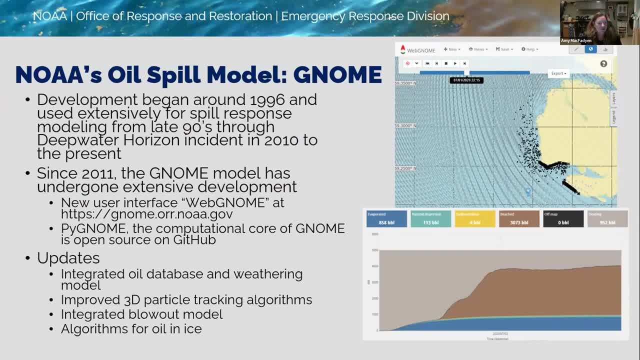 deepwater horizon, uh, the big, the oil spill in the gulf of mexico. the gnome model has undergone some pretty extensive development, um, in in the last decade or so. so that includes a new user interface, which is a web-based interface. it's publicly available, um. the url is there, and then the computational core. 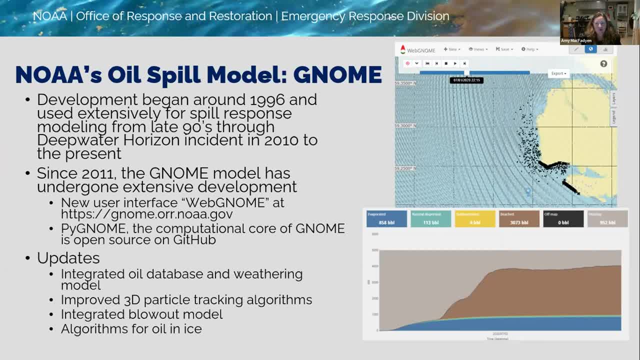 of gnome is. a is a standalone package. it's been separated out, which is is really useful for some of those more statistical applications that you might use for for planning um type type of modeling analysis. so we call that pinone because it's uh, it has a python scripting environment to access that. 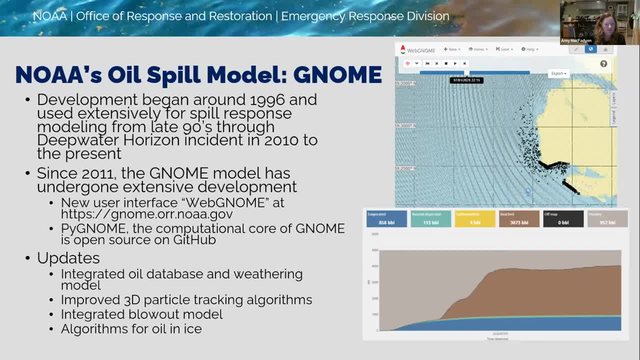 computational core and that is open source on github and publicly available as well, and we certainly welcome collaboration. um, i have some. the updates that i've listed here are not all relevant to this group, um, but the- the last one probably- algorithms for oil and ice we have. we. 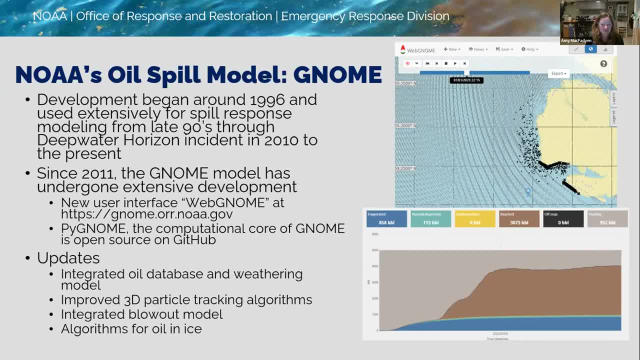 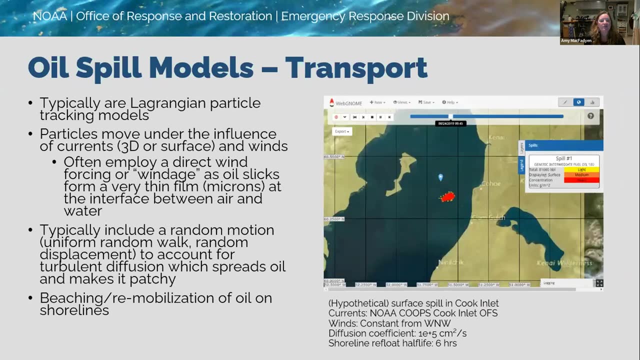 have added um in recent years some algorithms, some simple algorithms for oil ice interactions that we'll get to um a little bit later and in towards talk, i think um. so i did um because i don't know how familiar um the audience is with just oil spill modeling in. 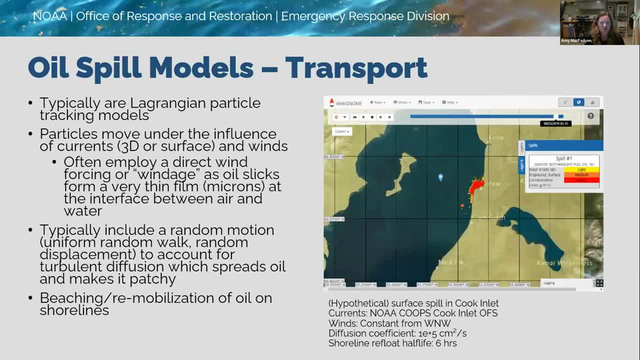 general, i thought it would be useful just to go over um kind of the general processes that are being modeled um in in- this is in in gnome, but also in general in oil spill models, because they they are similar in terms of the processes modeled um, even though they might be like a. 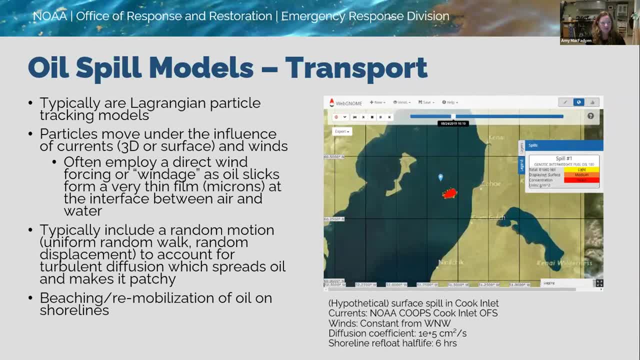 even if they might differ slightly in some of the algorithms, But typically we use the Lagrangian particle tracking approach for oil spill modeling, where the oil is divided up into particles that move under the influence of currents, either three-dimensionally or just surface. if we're modeling the movement of a surface slick, 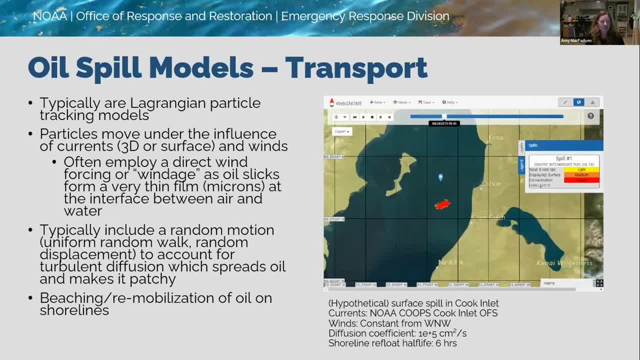 And also a direct wind influence is often used in oil spill models, And this is to account for the fact that the oil is basically in a very thin film at the interface between air and water, So it's kind of like a skin layer on the surface. 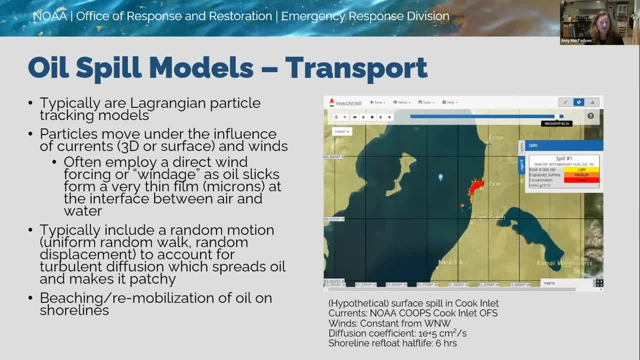 And because we tend to measure or predict models within about a meter layer at the surface. the oil is moving just right on the top, So we do basically a windage parameterization. that's generally in many models. somewhere around 3% of the wind speed is added as a direct wind effect. 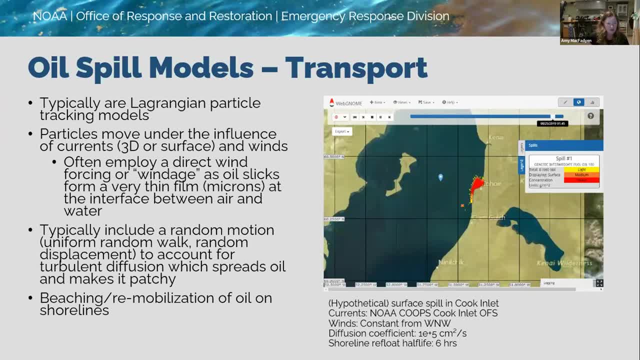 and it can have a rotation angle as well in some models. Oil spill models also generally include a random walk or sorry, a random motion, which can be done as a random walk or a random displacement model to account for the turbulent diffusion which spreads oil and makes it patchy over time. 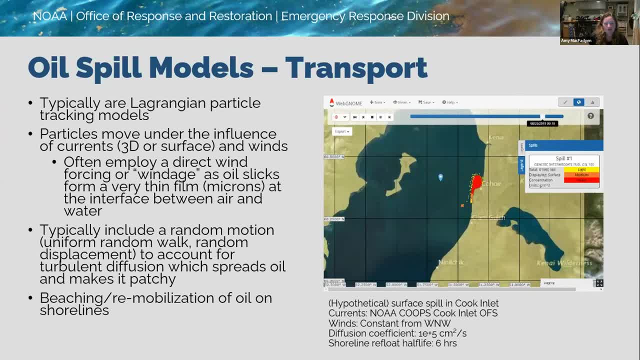 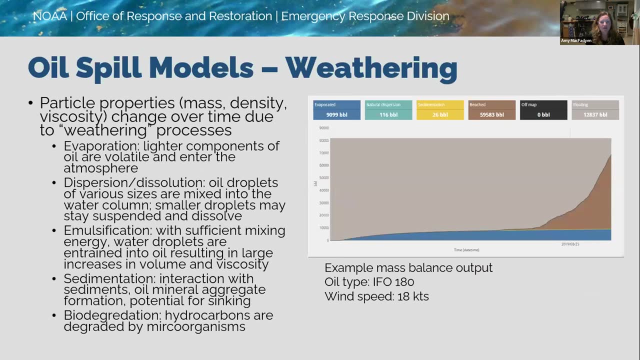 And then on the transport side, we also generally have algorithms for oil countermeasures, such as coming ashore, called beaching, and then potential re-mobilization of oil on the shoreline. The other processes we model are usually termed weathering. 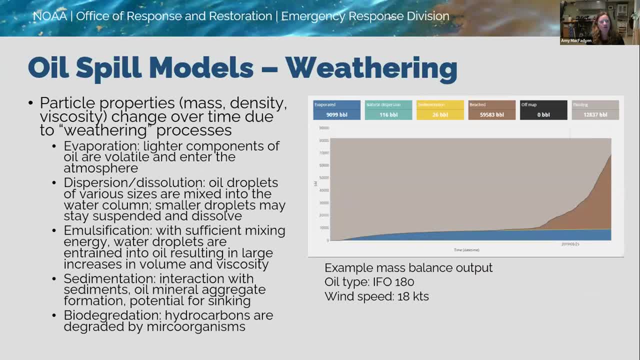 So these are biological, physical, chemical changes that the oil undergoes over time once it's spilled in the environment, And these basically change the particle properties, The mass, the density, the viscosity of the particles. So these include things like evaporation, where the lighter components of the oil are volatile and go into the atmosphere. 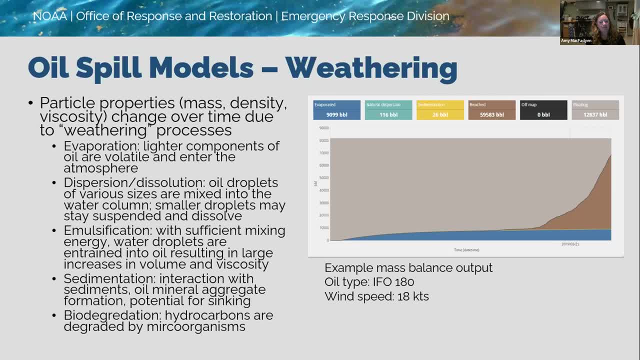 So this is a loss of oil from the ocean surface, But of course it could be a concern if those volatiles are concentrated enough where people are working on the response. We also include dispersion and dissolution. So dispersion is when oil droplets of various sizes 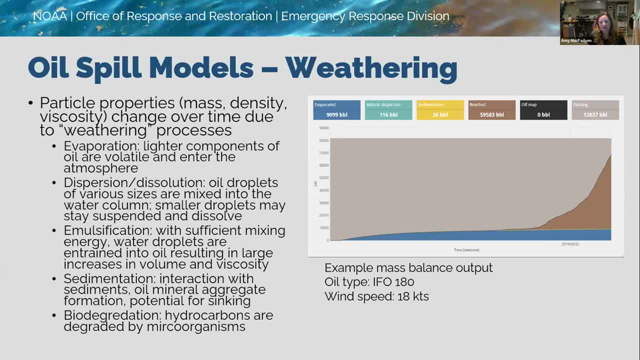 are mixed into the water column, The smaller droplets, you know. you make a whole mix of droplet sizes due to wave energy, and then those smaller droplets may stay suspended in the water column and ultimately dissolve, whereas the larger droplets might rise quickly and reform a surface slick. 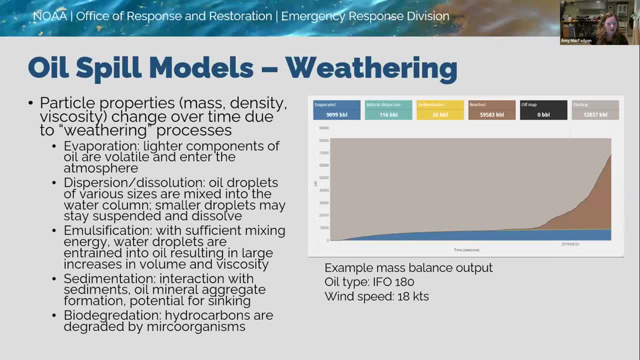 So that's included in Nome and other oil spill models. Emulsification is also generally included. The algorithms, I would say, are more. this is a very active area of algorithm development right now because it's a very hard process to predict, But with sufficient mixing energy. 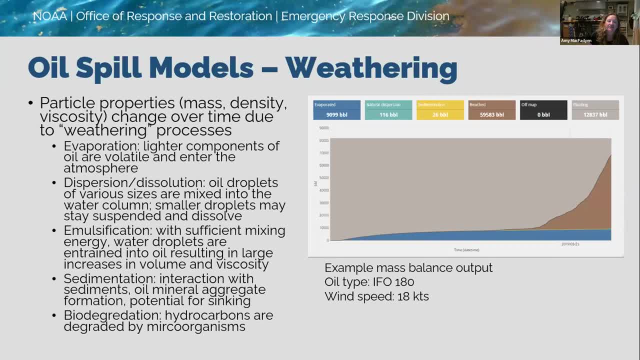 water droplets are entrained into the oil And this is important because it results in really large increases in volume, because you might have an emulsion with 80% water content, so it can radically increase the volume of material that responders are trying to recover. 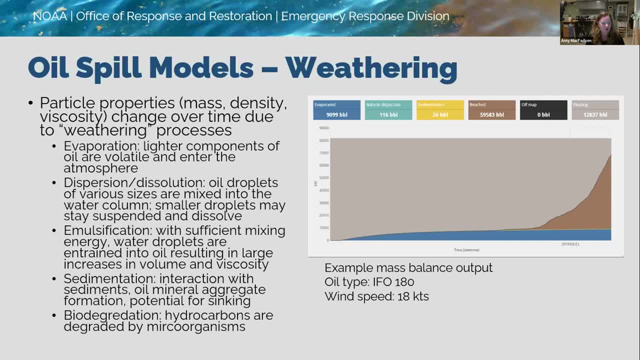 And it also has big implications. It has big impacts on viscosity, making the oil much more viscous, which also can be problematic for response. Sedimentation is another weathering process, or we term it as a weathering process, And this is just interaction with sediments. 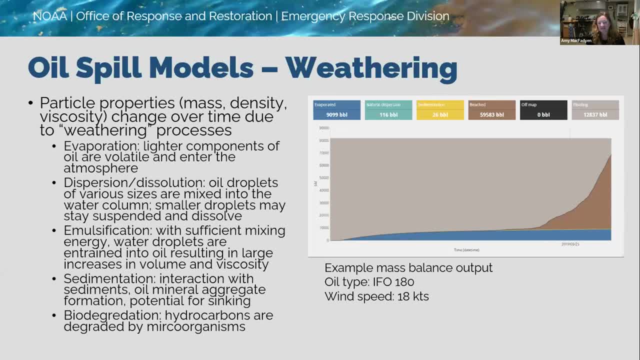 oil, mineral aggregate formation. And then there's potential, you know, in really in waters with a high sediment load, that you could form sinking oil due to these aggregations. And finally, biodegradation, in which hydrocarbons are degraded by microorganisms. 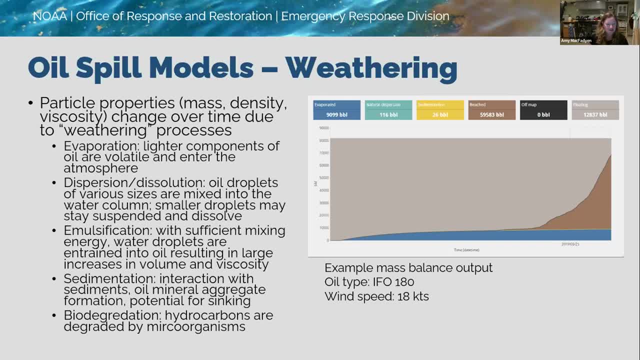 So this is a longer term process but can be, you know, the ultimate kind of fate of the hydrocarbons spilled in the environment And so on. the right picture is just kind of an example mass balance that you might get from an oil spill model showing the fraction of the spilled oil that evaporated. 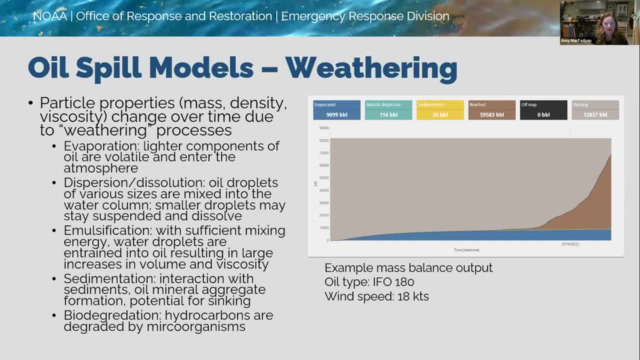 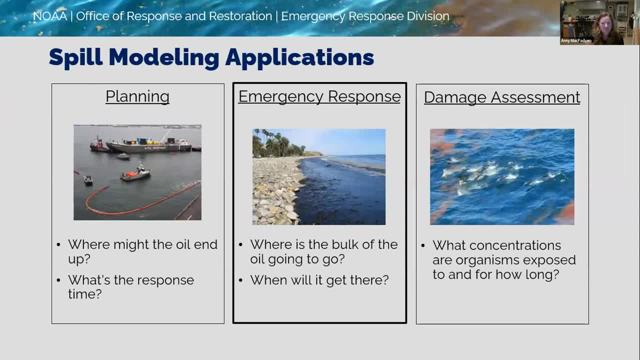 dispersed into the water column, formed aggregates, beached or remains floating on the surface. So I just returned to this slide because I you know I've been talking very generally about oil spill modeling, but I want to just focus now on. 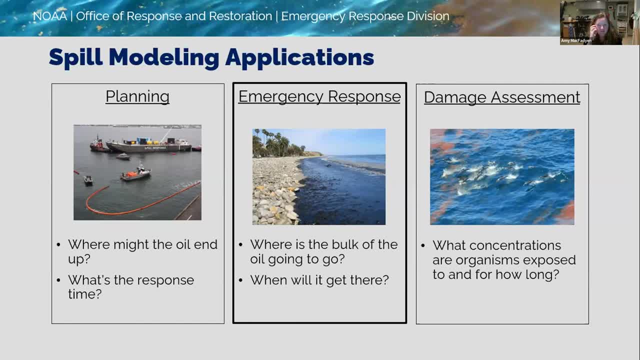 on emergency response modeling more, where the goal is really to provide a forecast that can be used to inform decision makers in a really timely manner, So with only the information relevant to the situation at hand. we want good information as quickly and simply as possible. 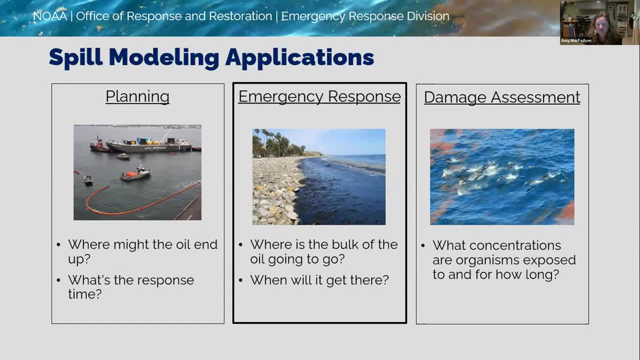 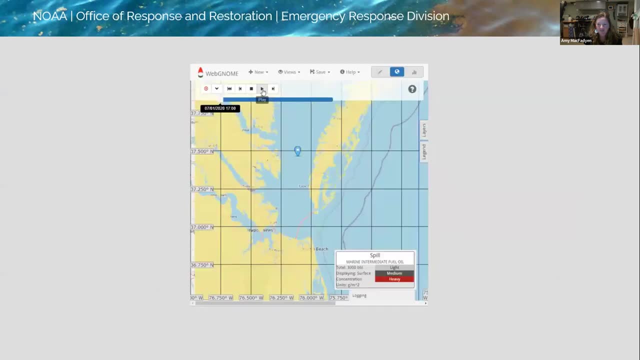 But of course, as an incident, there's a lot of uncertainty And so you know, as the oil spill model initially unfolds, there's often a lot of uncertainty in all the inputs to the oil spill model. So I think it's worthwhile to take a quick look at what goes into an oil spill model when producing oil fate and transport predictions. 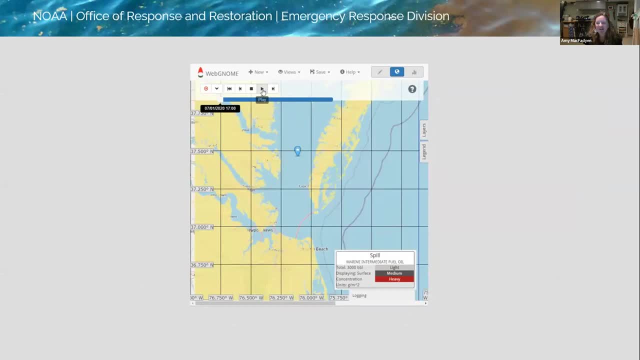 So here's just to start, a snapshot of our webnome model, because often we're talking about- you know, our spill model. I get asked: how accurate is it? Is it as good as so-and-so's model? Is it as good as? 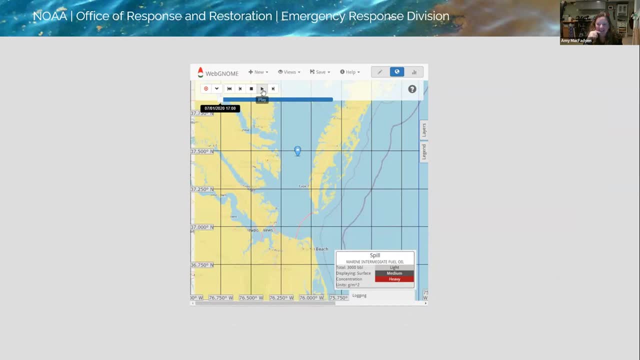 you know the model. Tor uses a Sintef model, And the answer, of course, is it depends. right, The unsatisfactory answer, But it does really depend And in particular when it comes to emergency response, the spill model is not typically the limiting factor in terms of accuracy. 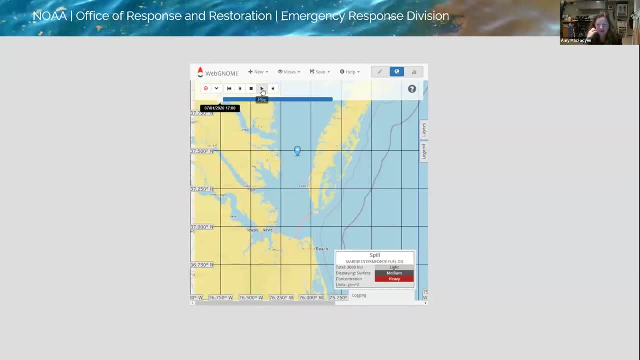 because there's so many uncertainties in all the model inputs. So really the question for emergency response is: is it useful? Does it inform the response with the relevant information that's accurate enough that they can, that it can support scientific supports, decision. 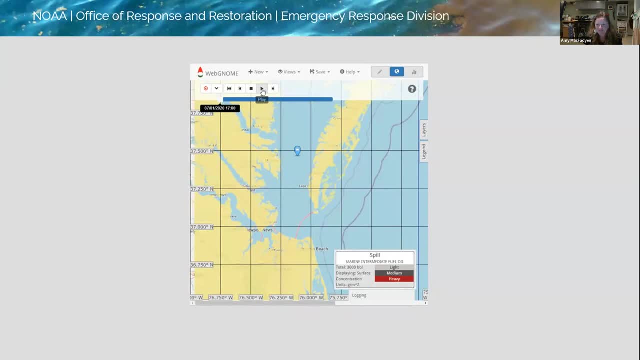 the decision making that needs to be done in order to respond to an incident. So what are these? I said I was going to talk about the inputs and the uncertainty associated with them. The first, most obvious input is: is what happened? What got spilled? 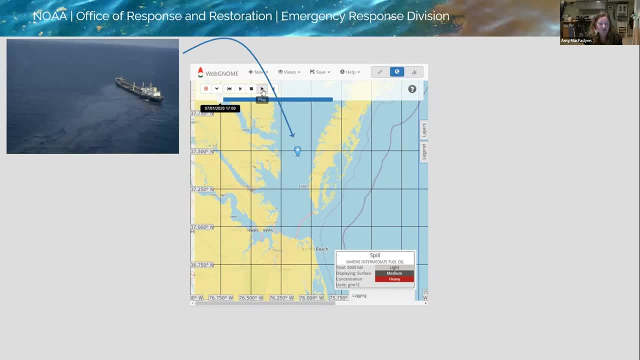 What's the product And what's the nature of the release. Is it you know? was it a point in time that it happened very quickly? Or is it a leaking pipeline? What's the location? And you know, having worked in emergency response now for 10 years. 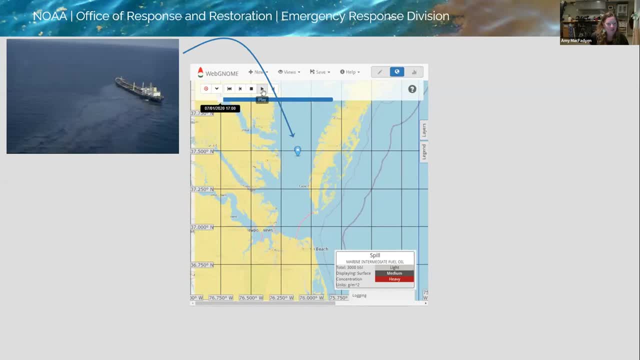 I can tell you that all those things that you, all that information you typically get on the first day, is much of. it is wrong. Even the location can be off. The duration is a big one that you generally don't know, Because 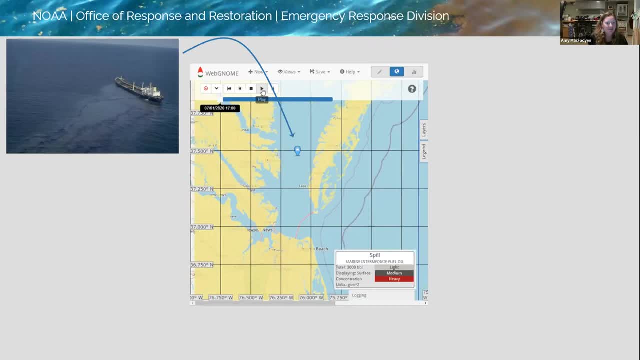 you know, some disaster has happened, whether it's a vessel sinking or a or a pipeline, And and there just isn't a lot of information about the details of of the release And and that really can make a difference. 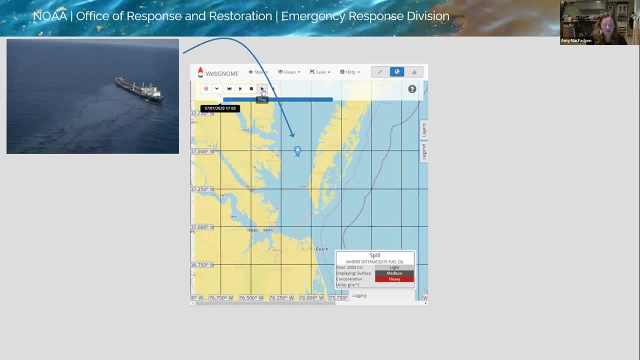 especially in in really tidally dominated waters where the currents are changing rapidly. If you release the oil- six you know- at one time and then six hours later you could get a very different, different result. So that's our first big source of uncertainty in emergency response. 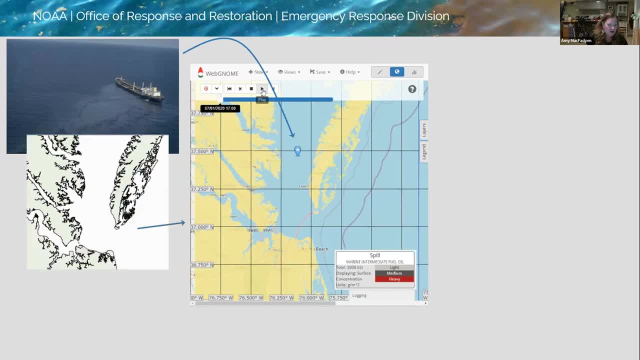 Modeling. We also need detailed shoreline in order to predict shoreline impacts. In general, that's not a huge issue, but there are parts of the of the U? S Coast that are, you know, rapidly changing, like Louisiana, for example. 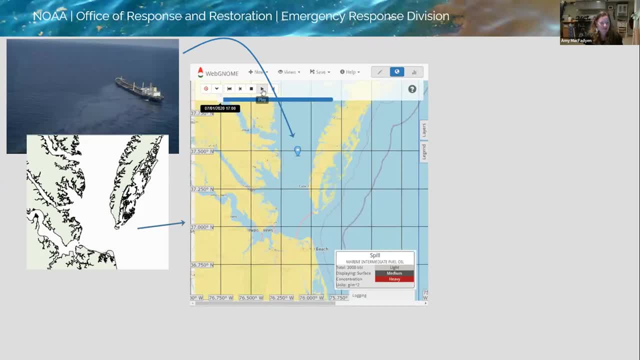 where it can be more problematic to know exactly where the where the shoreline is. Amy, I just I'm not sure how much further you have to go, but I want to make sure we have time for Torres presentation, So take it. 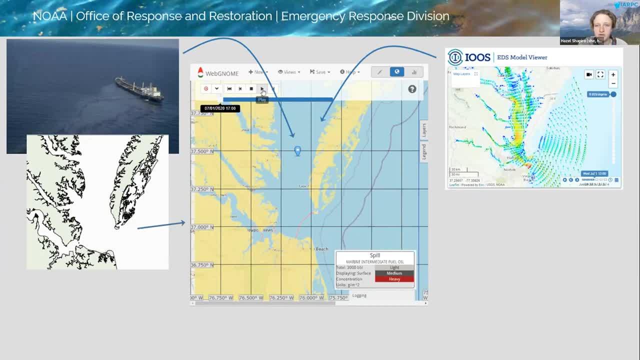 take a few minutes and but if you could go maybe more quickly through the last, Yeah, absolutely, I can wrap up pretty quick. You know, I'll just go through the rest of these inputs quickly, just making the point that you know. 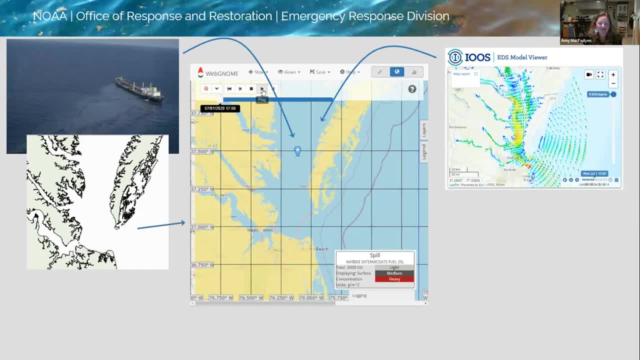 all of these, All the uncertainties that's that's going in, result to uncertainty in the output. So here's a snapshot of currents. Currents are generally coming from other hydrodynamic models which have their own uncertainties associated with them. So those are an input to the oil spill model to move the particles. 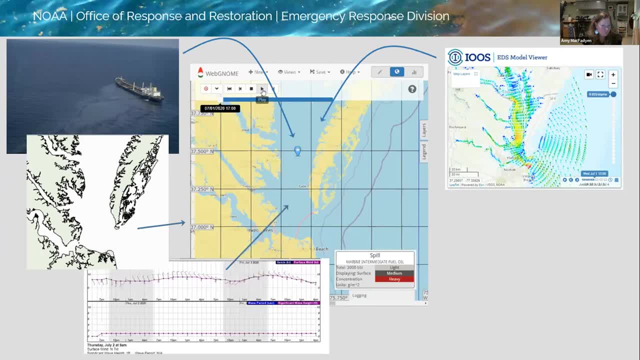 As our winds, which again are coming from. Usually our partners in the national weather service is where we go to for wins, but we all know there's uncertainty in the weather forecast And the The last picture that I have there is this of observations: 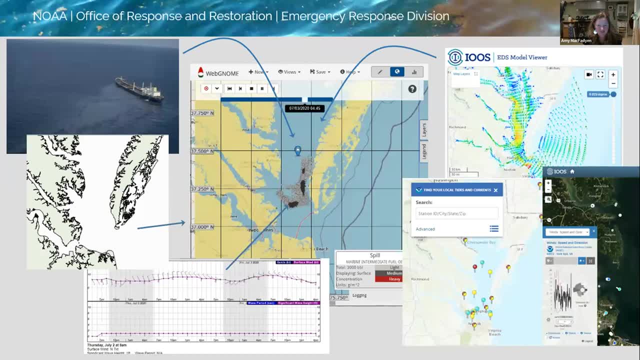 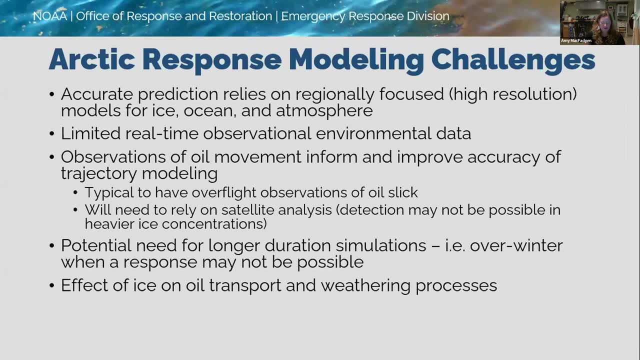 which can be used to kind of constrain and reduce uncertainty. If if we want to make sure that the knowledge is available, it's probably not too surprising. If we want to make sure that the spatial observational data is available, we can use it to validate our inputs. 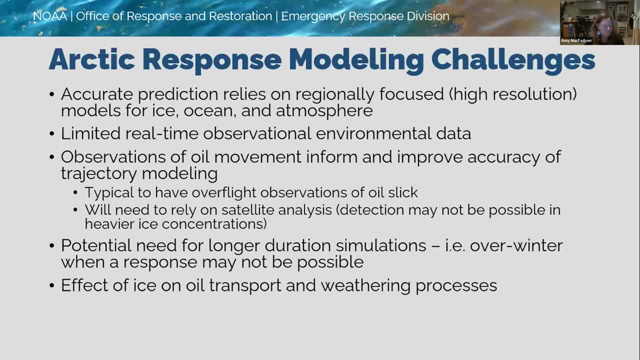 So all of these Inputs You can, it's probably not too surprising that if things are exacerbated when we come to the Arctic, The you know. so the first few challenges that I've listed here are fairly obvious. Accurate prediction relies on regionally focused 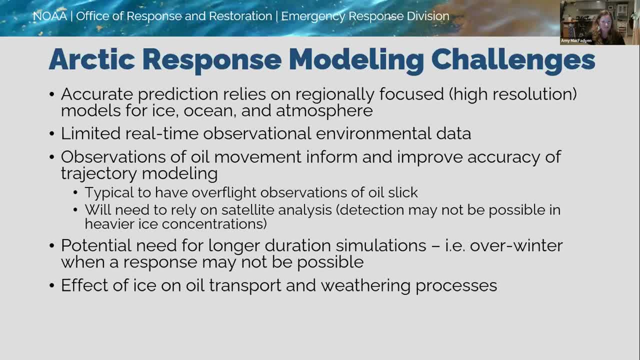 be inputs to the oil spill model, which would be not readily available for the Arctic. We also have limited real-time observational environmental data. The observations of oil movement are really important to improve the accuracy of trajectory modeling, because we usually don't, as I said, 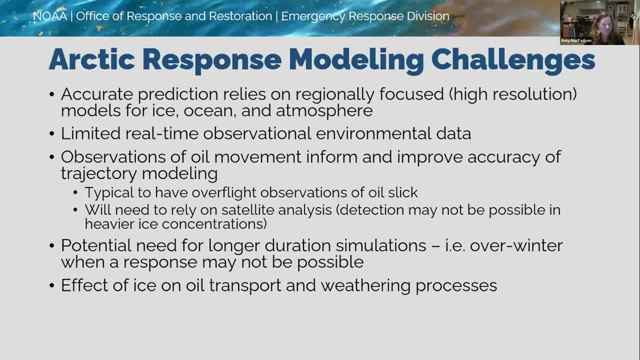 we don't know a lot about the release information, So we typically deploy people to fly over the slick through helicopters or drones, now increasingly, to give information about the extent of the oil slick and how it's changing, what it looks like, And that feeds into the model. 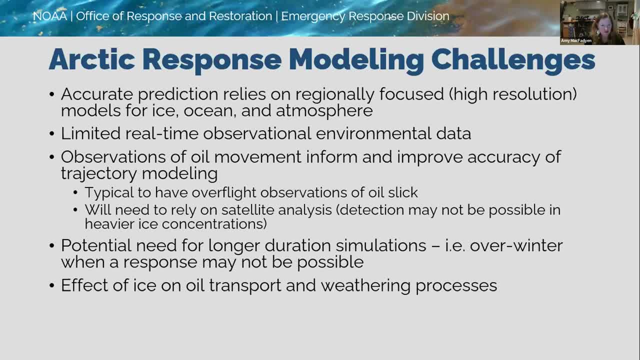 and it's unlikely that we would get those observations in the Arctic at all, or not in a timely manner, And so we need to rely solely on satellite analysis, which has its own issues with detecting oil in heavier ice concentrations. There's also in the Arctic, I think, a potential. 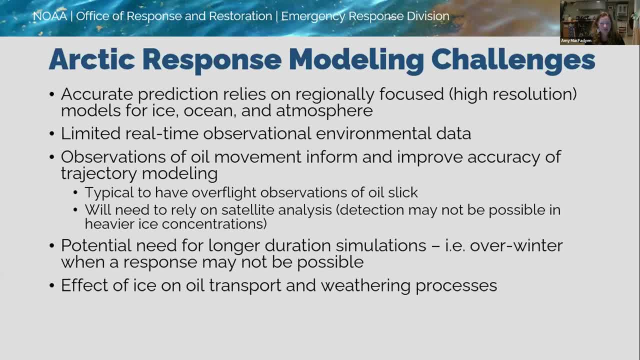 need for much longer duration simulations. The response time is going to be slower to get you know if it is feasible to respond. getting people there will take longer. And then there's a potential for needing to model over, you know, over a season, if a response is not possible during the winter. So predicting what? 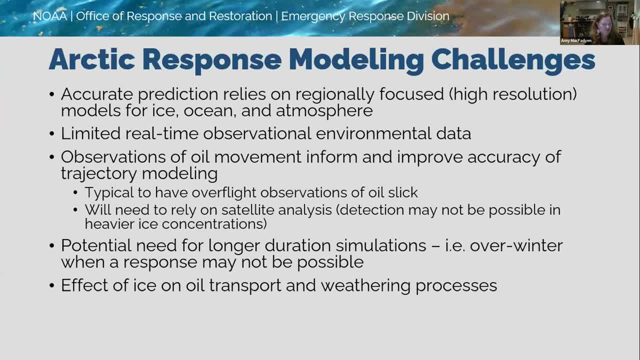 might happen over these longer timeframes is a big, you know a particular challenge. And then finally, of course, the effect of ice on oil transport and weathering process. So ice makes a big difference to all of those processes that I outlined earlier, on both the transport. 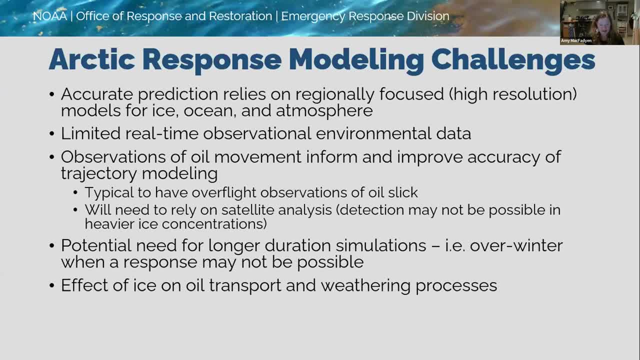 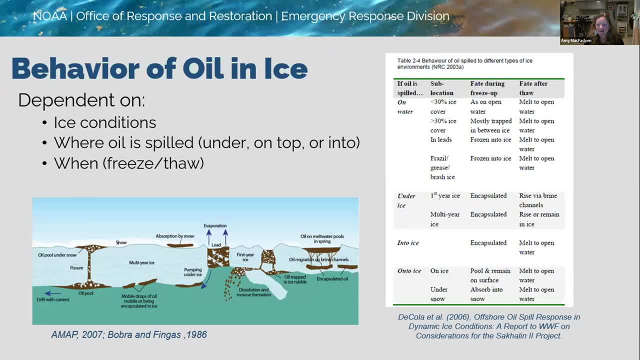 and the weathering side. there's impacts And I'm hoping that Tor is going to go into that. since I do not have time, But I will just leave with this slide. perhaps that just shows you know that the behavior of oil and ice is very complex And we certainly 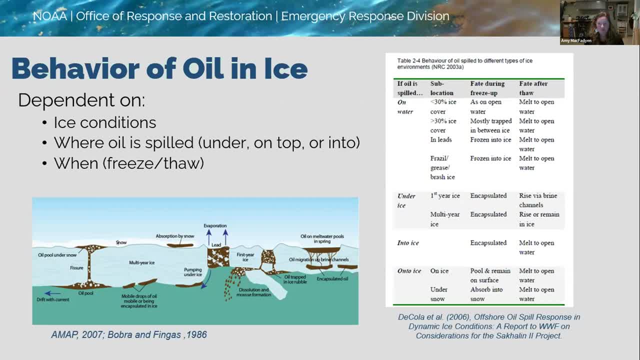 don't have the ability to model the physics of ice movement and formation on the scales that are really relevant to oil ice interactions. A whole variety of things can occur depending on, you know, the ice conditions. the percent coverage will be a big factor in how the ice 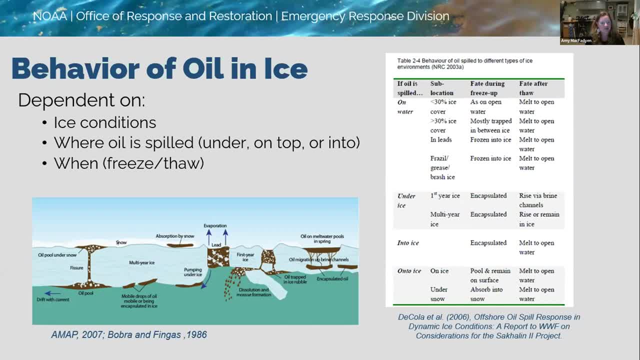 moves. If it's, you know, below some threshold, then the ice might just, or the oil might move as it normally would in open water, Whereas if it's above some threshold, the ice could, the oil could become encapsulated in the ice and move with the ice. Where the oil is spilled is also important. 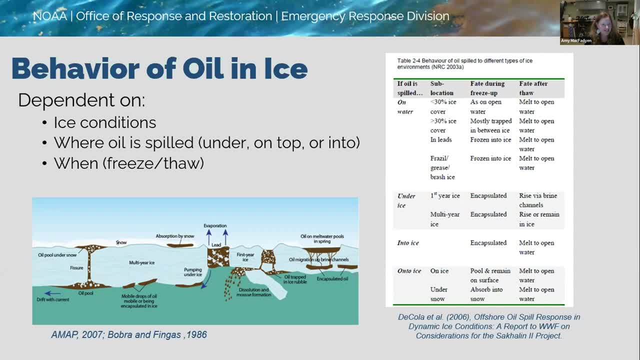 whether it's spilled on top of the oil, ice under the ice or into, you know, broken ice will affect what happens. And then the seasonality is super important as well: If is the ice freezing in a freeze Period of time or is it thawing, And that's going to make a big difference in the oil. 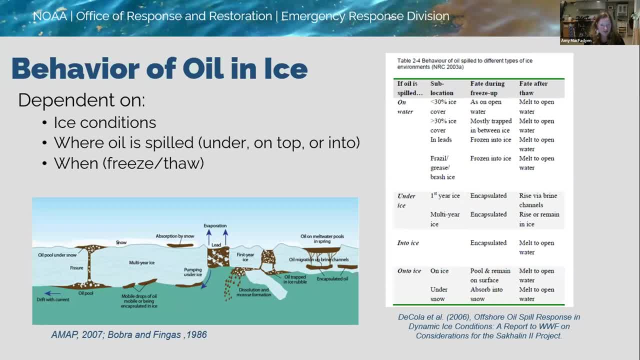 in the oil fate. So I think, in the interest of time, I will just stop here because I'm, as I said, I think TOR is going to take up the oil ice interactions topic in more detail. Great, Wonderful. Thank you, Amy. That's very, very interesting. I'm sorry we're running. 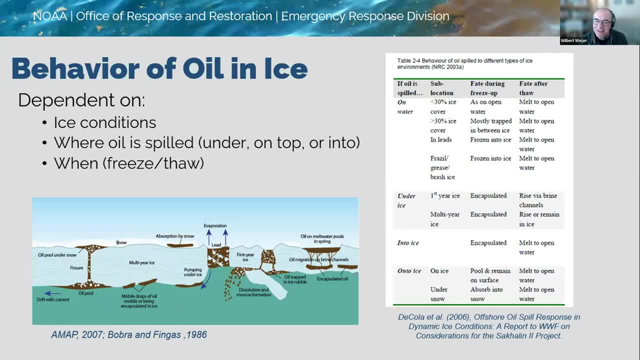 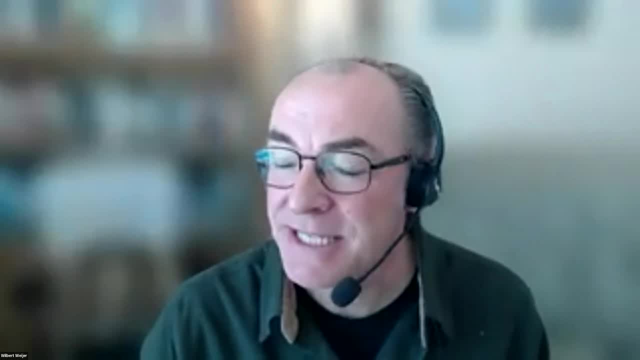 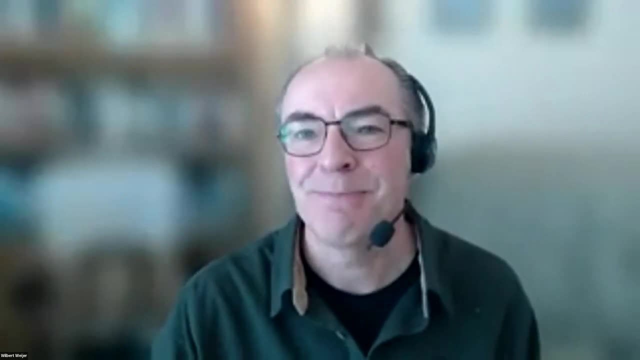 a little bit bit late here, So if we have some time for questions later, then we'll. I will get back to you, But let's, yeah, and please ask questions and answer questions if you can in the chat. that would probably be. that's perfect, And so maybe we'll hand it over to TOR. Thank, 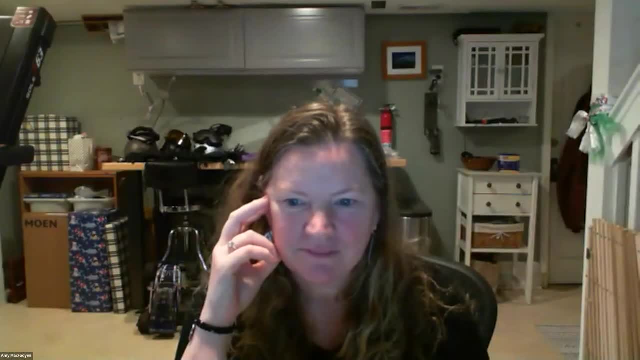 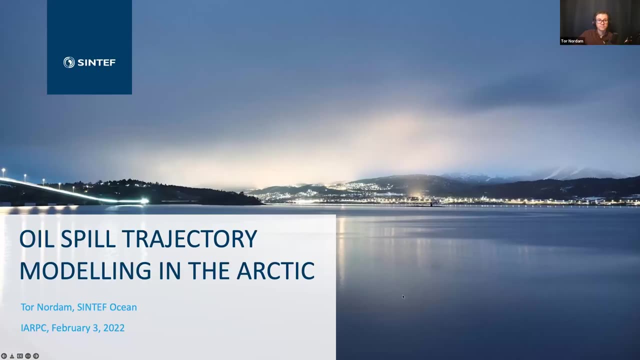 you very much, Amy, Appreciate that. Not a problem, Really, really nice. All right, Can you all see my slide and hear me? Yes, sir, Yeah, perfect. So I keep getting messages from Zoom saying: yeah, my internet connection is unstable and sometimes the sound drops out for me. 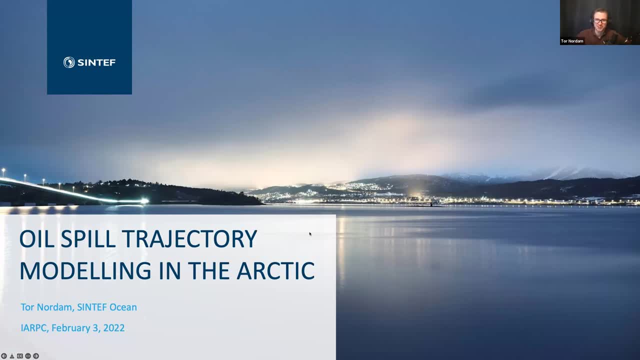 So if you can't hear me or if, then please let me know and I'll try to repeat. So, as I said before, my name is TOR Noram. I work for Sintef Ocean, which is like a nonprofit research Institute in Norway, and Sintef has been involved with- I mean Sintef does- many. 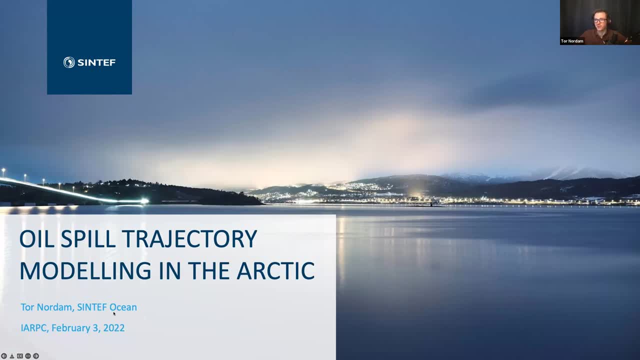 things, but there is at least a department that is currently known as the department for climate and environment, And people in this department have been working with different aspects of oil spill research for something like 40 years, i think. um, yep, so i'm- yeah, i'm- a physicist myself. um, i'm going to talk about, or a computational physicist. 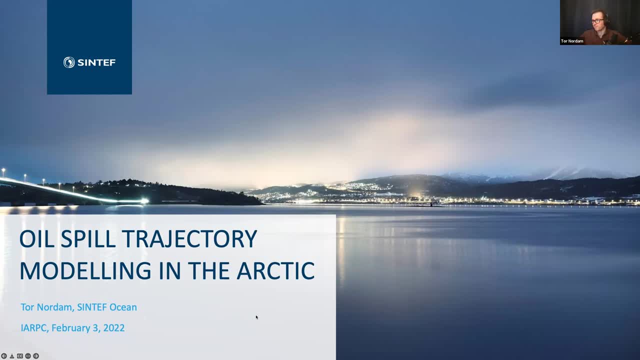 and i will talk about, um, the modeling of oil spill, oil spills in arctic, and my outlook is, it is um a little bit more theoretical. maybe, um, there is nobody who's going to use, or i'm not going to tell anybody where they have to be- in like six hours with the booms. i'm talking, i'm thinking. 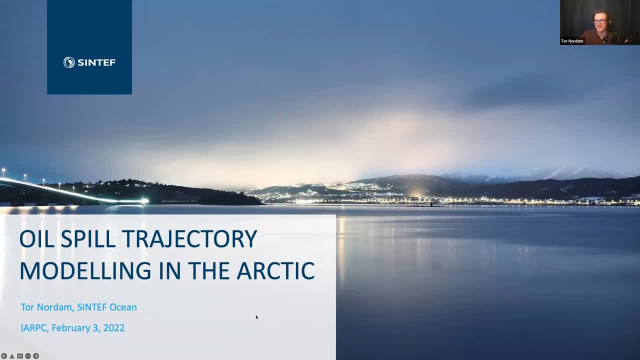 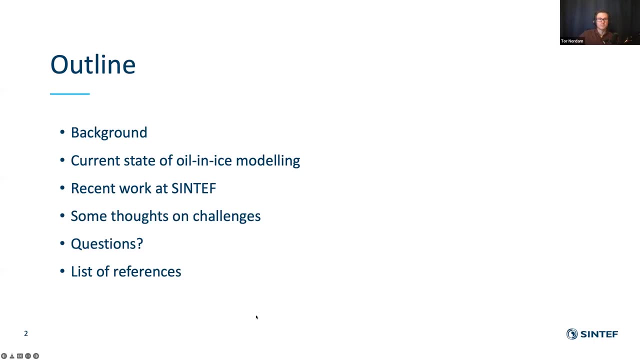 more about, uh, things like risk analysis ahead of time, i guess, and um development of models and and so on. um outline of my talk is that i'm going to talk a little bit about background, then i am going to describe what i think is more or less the current state of the art in oil and ice modeling. 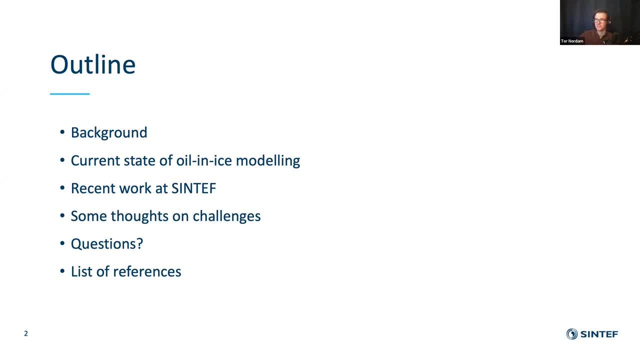 now i'm going to show a few examples of recent work we have been doing at Sintef. i will share some of my thoughts on a couple of challenges that i see with oily nice modeling- not necessarily the biggest challenges, but at least two challenges that i have been thinking of um. 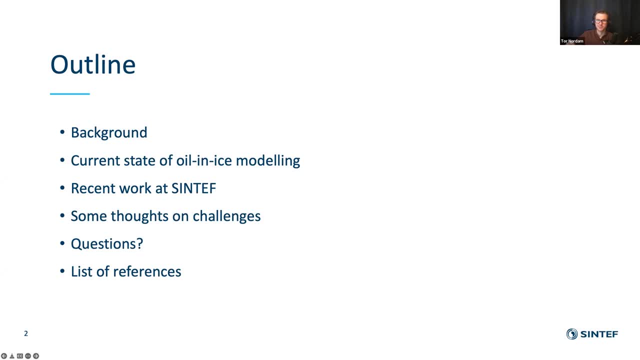 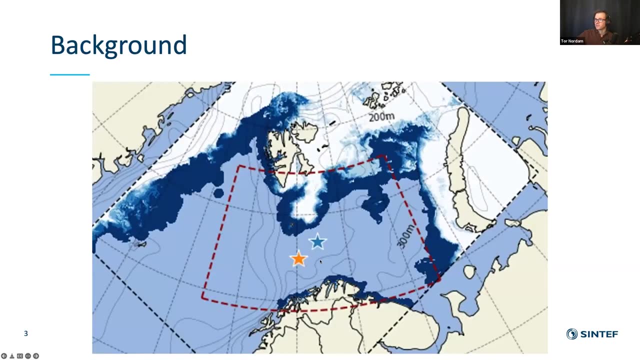 and maybe we have time for some questions at the end. and if you download my slides, which i think will be shared on the internet, then you will find the list of all my references at the very end. so just to open up with this picture. i think certainly in norway when people talk about 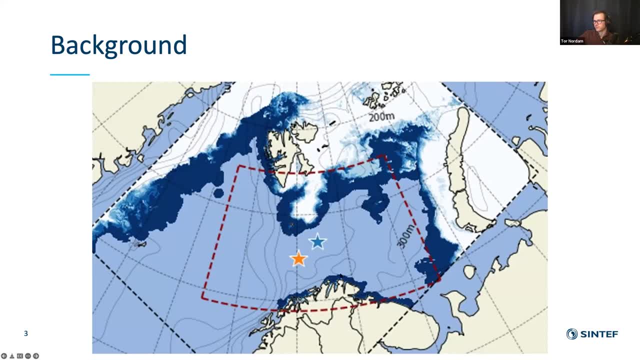 oil spills in ice. this is kind of what people think about. so this is northern norway, right here um. oslo is far to the south, outside of the slide, and these two stars represent what i believe are the two northern most oil developments currently ongoing in norway. and this is svalbard up here: sea ice. 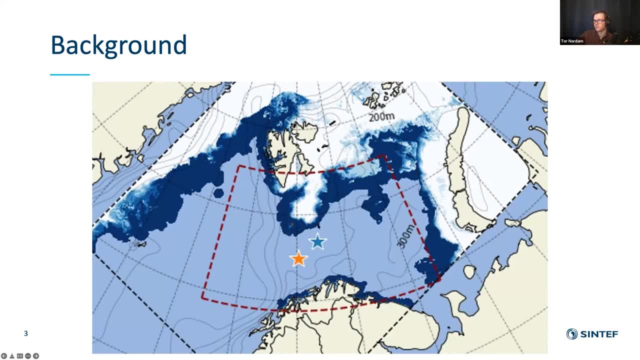 here. this is, i guess, about as far south that the sea ice currently extends um, and when people think of it they may be a bitже FR kdc science, i think here is guys talking about- and all these bell INE on that up về smilnge dressed for a board meeting in norway for three months in Norway. 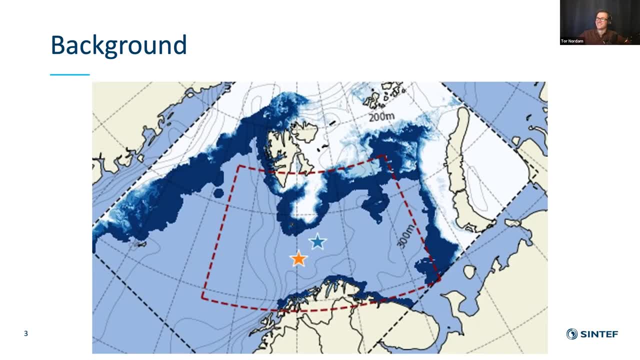 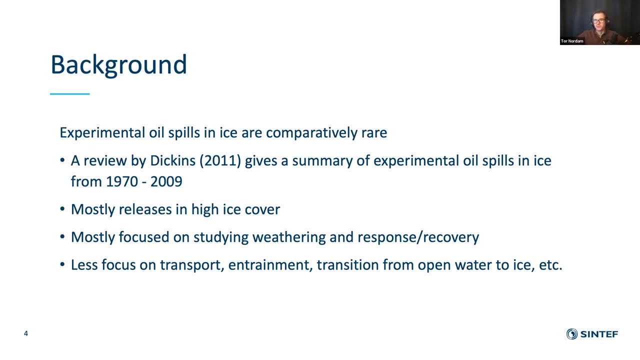 that. but anyway, this is, um, this kind of picture is one of the reasons, i think, why oil spills in ice have received a bit of research funding. um, you know right, yeah, um, some of what we do know, or i guess, yeah, i mean some of what we do know from about oil spills in ice, we know from actual 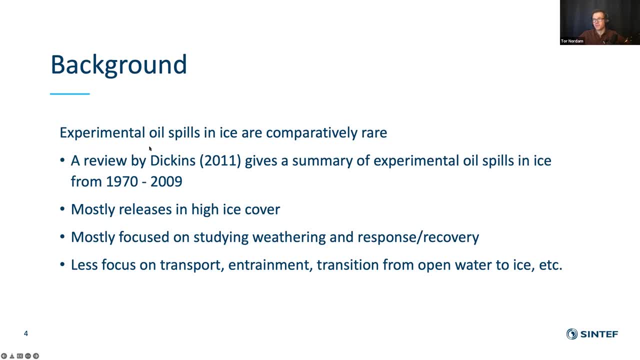 accidents that people have observed and some things we know from experimental oil spills in ice. however, experimental oil spills in ice, they are rare compared to experimental oil spills in the field without ice. um, and a lot of these releases they have been done in high ice cover and they have focused mainly on either how the ice affects the weathering of the oil or how it 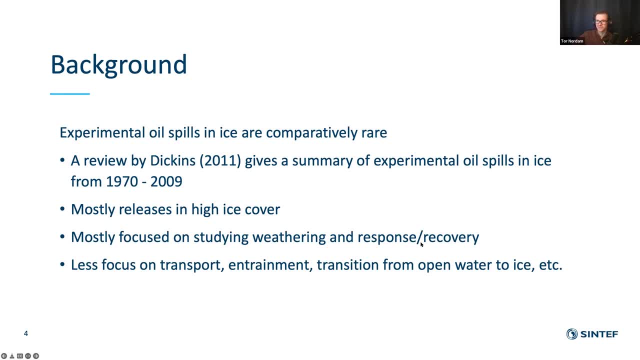 affects response and recovery. so people test different skimmers or they test in situ burning or things like this. they've been less focused on things like transport and trainments and the transition from open water to ice. so what happens if you spill a lot of oil in open water and it? 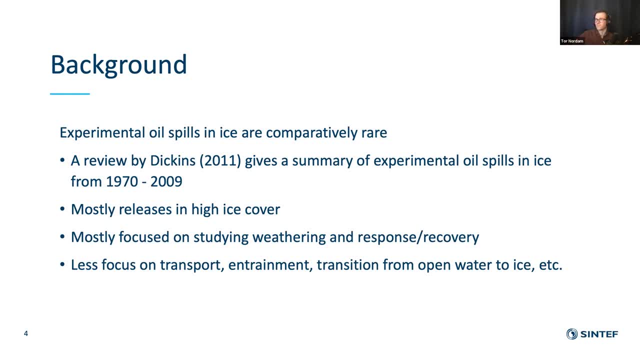 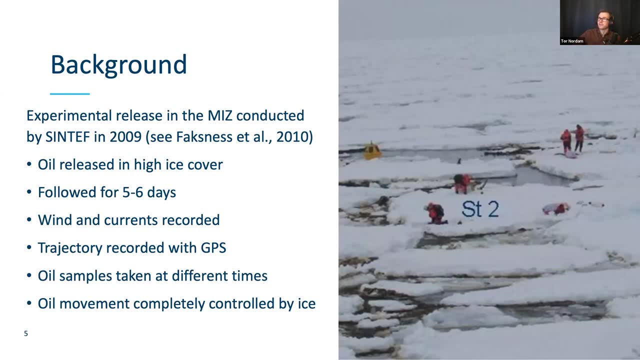 kind of drifts into the marginalized zone and starts mixing with ice. um. this is an example of one of those experimental oil spills in the field. this is a field study that was done by Sintef in 2009, so that's before, before i joined Sintef um, and you can see here. 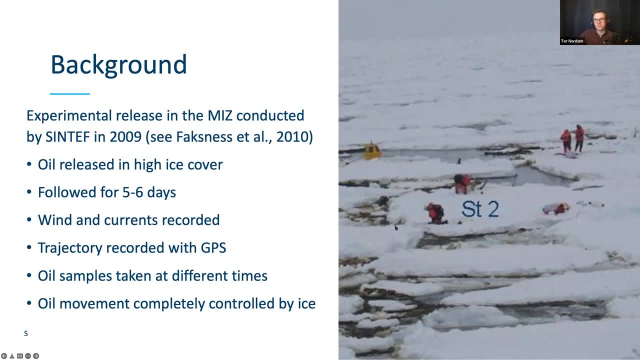 there is some oil in between the ice flows here. so this was oil that was spilled in the marginalized zone in very high ice cover and it was trapped in a very high ice cover and it was being tracked for about five days and they measured the winds and currents and the 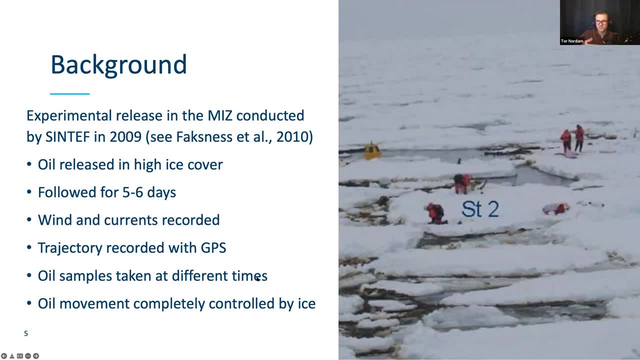 trajectory was recorded with gbs and so on. oil samples were taken at different times to say something about the weathering and composition of the oil. sorry about that, i clicked the wrong button and um from this experiment- unsurprisingly, i would say- they found that the oil movement in a case such as this is completely controlled by the ice. 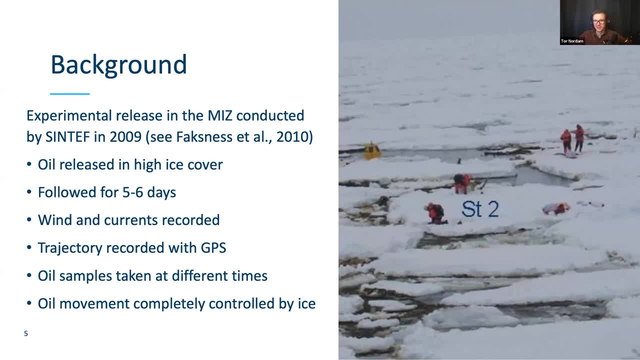 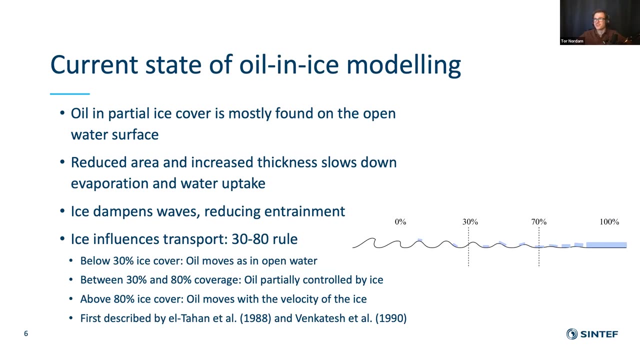 because i mean, here you have probably something like 90 ice cover and basically all of these ice flows are touching, so there is no way that this oil is going to move in any way different from what the ice does. yeah, um, just to kind of summarize what i think is the current state of 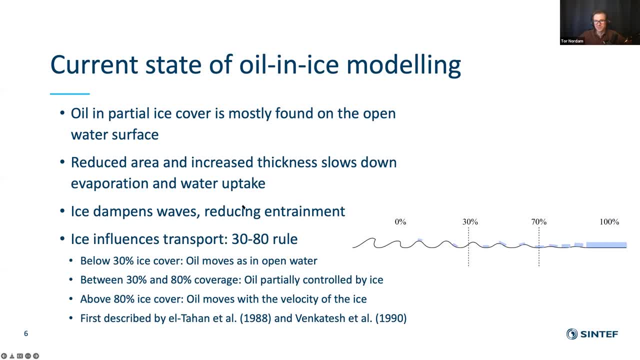 the art in oil spill modeling. um, what do we actually know and what is actually implemented in oil spill models these days? so we know that when you have partialized cover, then the oil is going to more or less collect in the, in the leads and the open water between 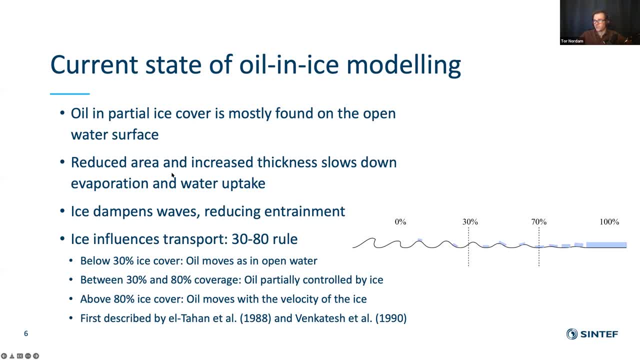 between ice, and this, of course, reduces the area that's available to the oil and it increases the thickness, and this again slows down processes like evaporation and water uptake that are dependent on the interfacial area between the oil and the ice and the atmosphere, or 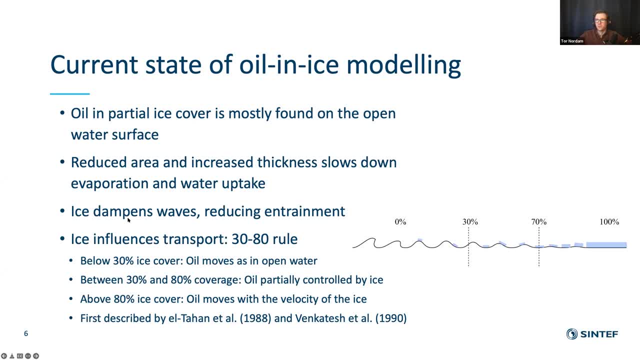 on the water in the atmosphere. ice will also dampen the waves, which reduces entrainment of oil and ice influences transport. amy mentioned this. you have something called the 3080 rule which says that if you are below 30 ice cover, then the oil moves as in open water. if you are above, 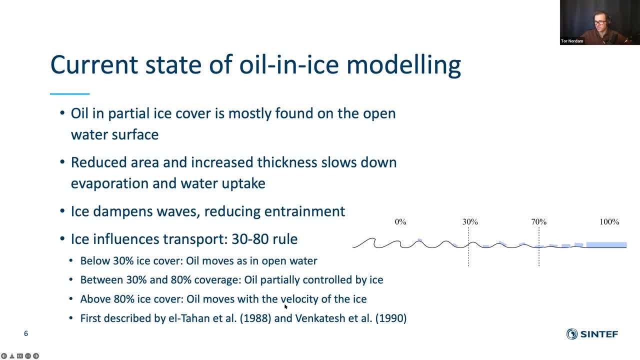 80 ice cover, then the oil moves with the ice and in between you have something in between not specified too closely. i believe this was first described in a technical report, which i have been unable to find so far, from 1988, and then some other papers from around the same time by some. 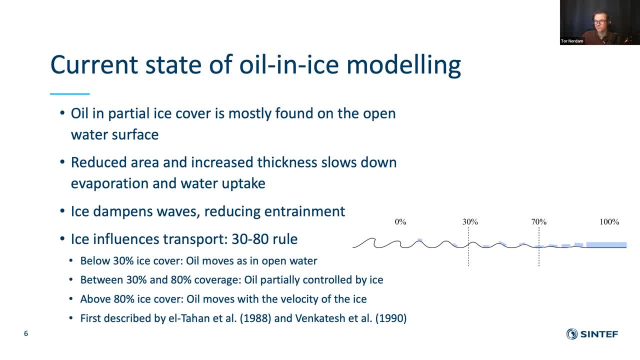 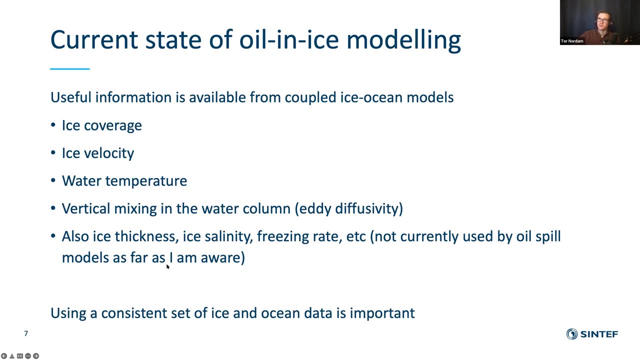 of the same authors talk about this, but it's kind of based on a few observations of accidental oil spills as far as i know, and it's so it's not super well funded theoretically this stuff, but but this is implemented in oil spill models nowadays. you can also get a lot of useful. 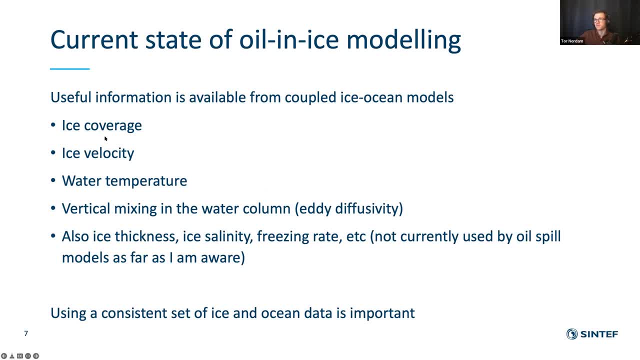 information from coupled ice ocean models, things like ice coverage, ice velocity, water temperature and the vertical eddy diffusivity in the water column, and all of these are also used in oil spill models. ice ocean models also predict a few other things, such as ice thickness, salinity, freezing rate, etc. and, as far as i know, this isn't used by oil spill models. 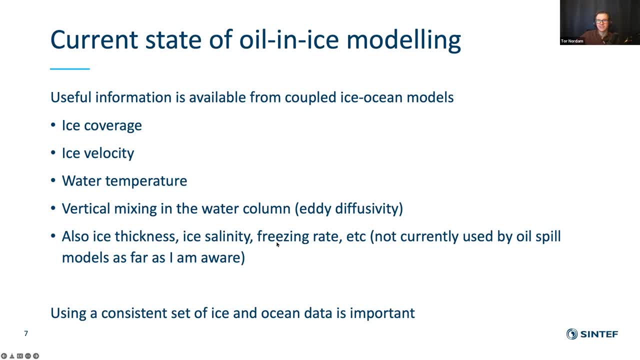 although i could be wrong, and i guess things like freezing rate could be very useful, because you could think about oil getting frozen into the ice and then being released at some later point then. so, yeah, anyway, useful information is available from ice ocean models and it's important when you use. 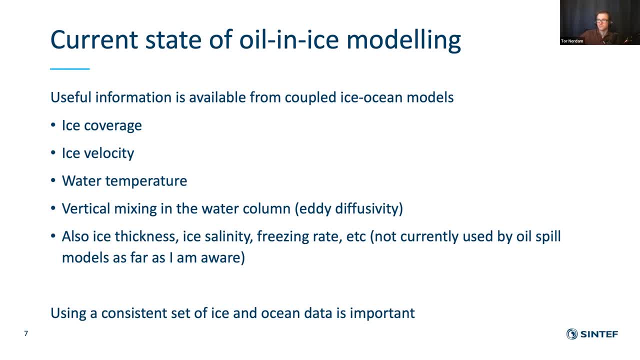 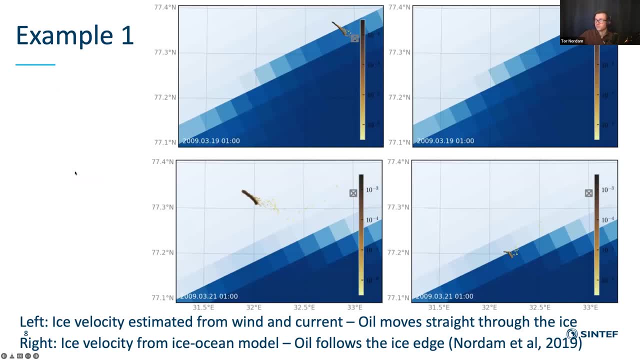 these models to use consistent set of ice data and ocean data and so on. so i'll show an example of that. this shows a hypothetical release in the marginalized zone north of norway. and there is this: this gray square here shows the release site. and on the left here this is soon after the release. 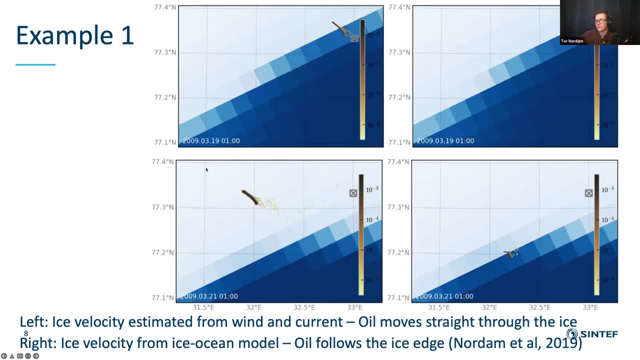 and this is a bit a couple days later. on the left i have used current and wind, but then i have used an ice velocity which is estimated from the current element, and then what we see is that the aisle and the the oil that's released, it kind of moves straight in through relatively high ice. 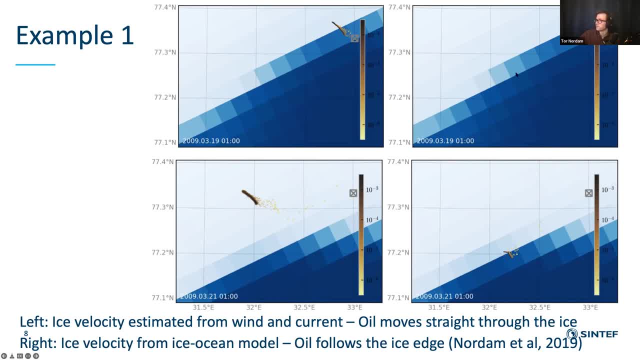 cover, which is contrary to what you'd expect. on the right, i have done the same simulation, but i have used an ice velocity that comes from the coupled ice ocean model, so it's a nice velocity that is consistent with the currents and the wind, and in this case you see that the and. 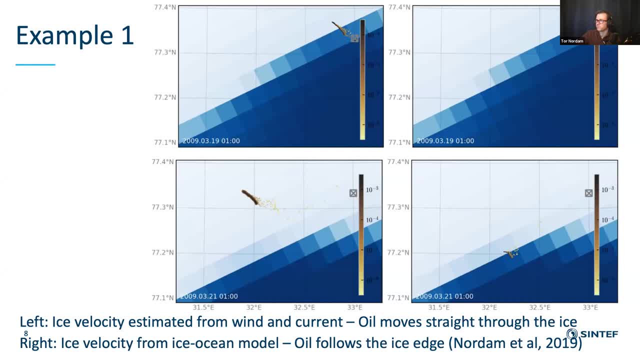 additionally, in both of these cases i've used this 3080 rule that i mentioned previously. um, so in the two pictures on the on the right here, you see that uh, some days after the release, the oil still remains uh kind of on the border between or in in the marginalized zone, basically. so this: 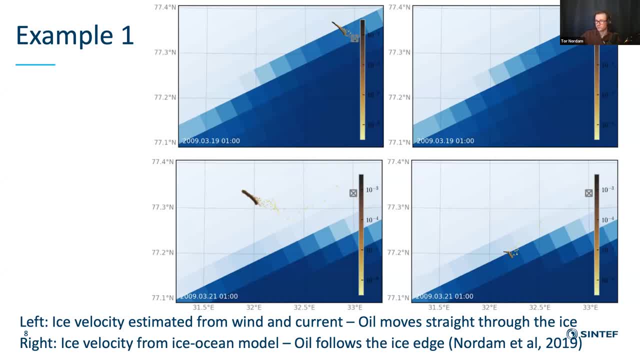 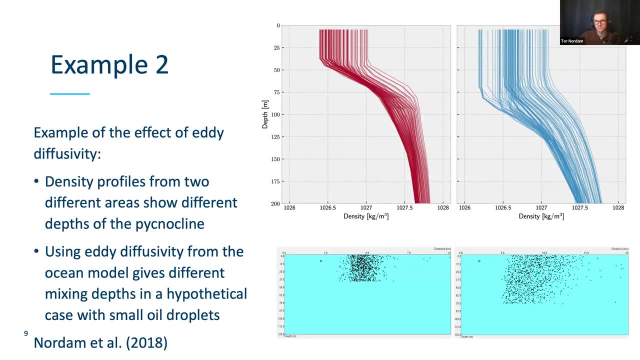 is just a hypothetical case, but at least it seems much more physically reasonable when you use a consistent set of data. this is another example of using data from a coupled ice ocean model. this top panel shows shows two different sets of density profiles from two different areas. so on the left you have the depth of the pycnocline is at something like 40 to 50 meters. 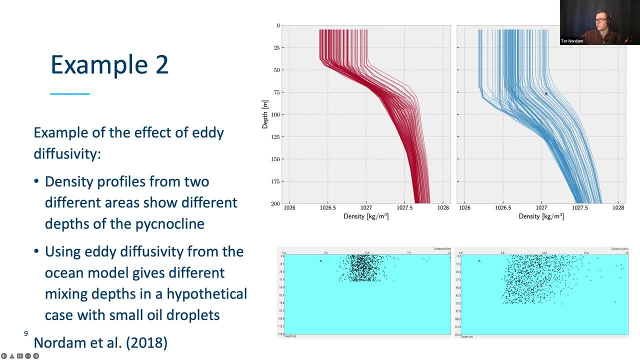 and here on the right you have a pycnocline that's at around 75 to 80 meters and this is going to affect the vertical diffusivity. so the mixing, because in the top here, where the density is constant, you have much higher vertical mixing than you have. 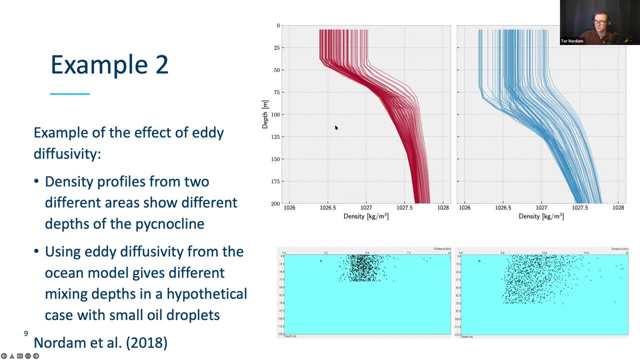 once the density starts increasing, and if you use this as input to an oil spin model, which is what we see at the bottom here, then this affects how deep down the oil gets mixed. so this is it's again, it's a hypothetical scenario where i've released the really tiny oil droplets that 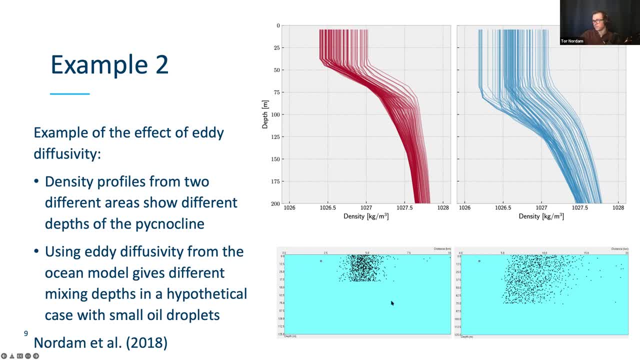 mix quite quickly. but but you see the difference in using using this information from an isocial model. so of course you can ask: is this model going to be right? um, that's an important part of the uncertainty, but at least that information is there and, um, yeah, it might be worth using it. 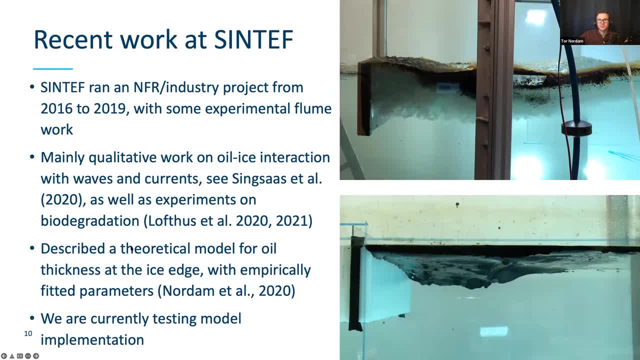 if you're not sure if it's working or not, but it's a good idea to check that out. to mention some recent work we have done, at Sintef we had a project that ran for three years, from 2016 to 2019, where we did a bunch of experimental work, in some flume work, and 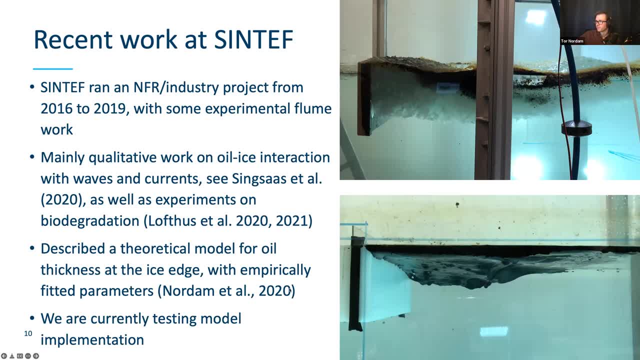 some other lab work, for example on biodegradation. there are a couple of references here, and we also looked a little bit at what happens when current forcing oil on the surface towards an ice edge, or i guess in this case it's a- technically it's a polypropylene edge, but the point is that the oil kind of gets compressed. 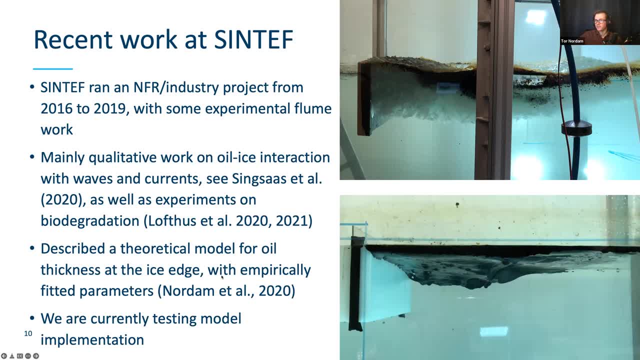 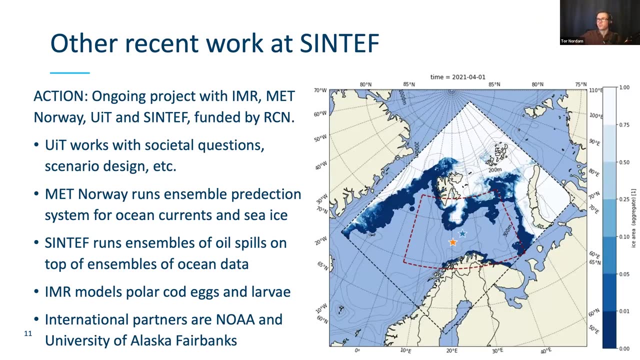 when it's being pushed against ice action. yeah, um, currently we are testing some model implementations of this thickness model and also some of the biodegradation data that was received from or derived from this project. other recent work at Sintef is an ongoing project that we have together with 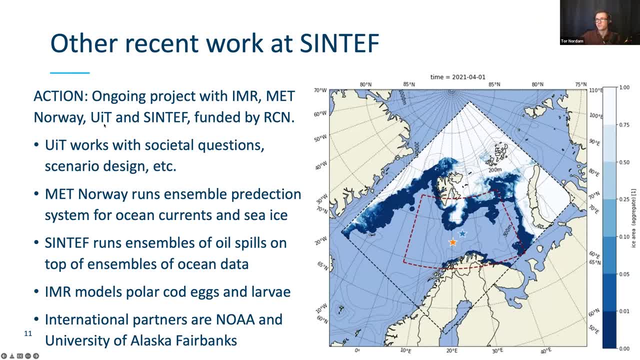 the institute of marine research in Norway met Norway, university of Tromsø, Sintef and international partners, NOAA and university of Alaska, Fairbanks. this is, i think, a quite interesting project. university of Tromsø: we have sociologists who are talking about social questions and fisheries and things like this. then met Norway, runs an. 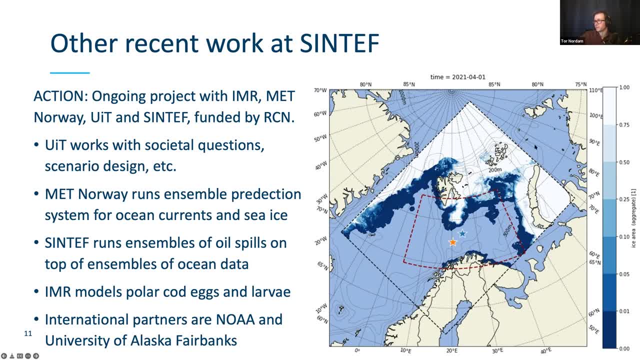 ensemble prediction system for uh, this area here where they look at currents and sea ice, and then Sintef is going to run ensembles of oil spills on top of those ensembles of ocean data to get statistical predictions of what might happen, and then the institute marine research is going to run their 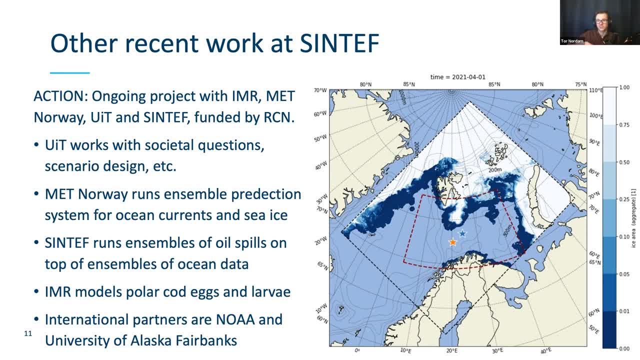 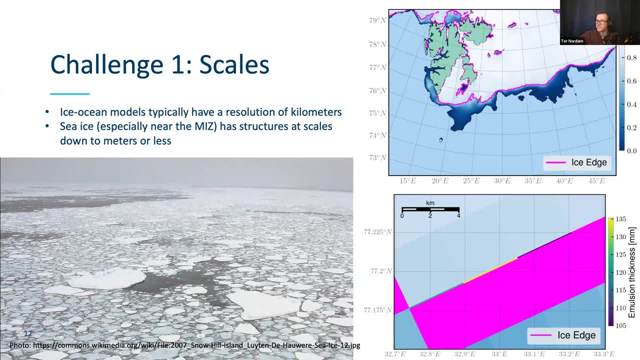 model for polar cod eggs and larvae to look at potential impacts of an oil spill. to mention a couple of challenges that i see with improving oil in ice modeling. Amy has already mentioned the scales. on the left here we see a picture of sea ice. this is actually in the antarctic, not the arctic, but 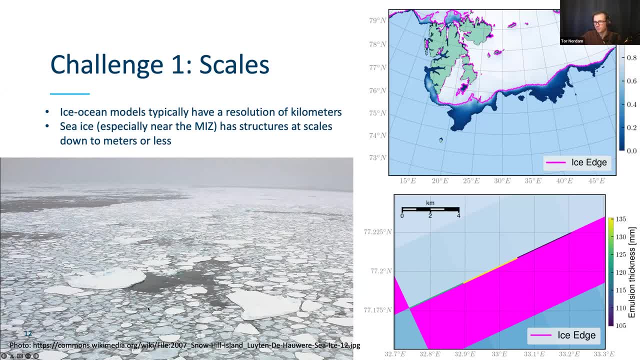 still, there is things here going on down to meter scale and even smaller, and on the right you see examples of ice model data where you see the ice edge here and zoomed in on the ice edge here, and each of these squares are four by four kilometer and you don't know anything about. 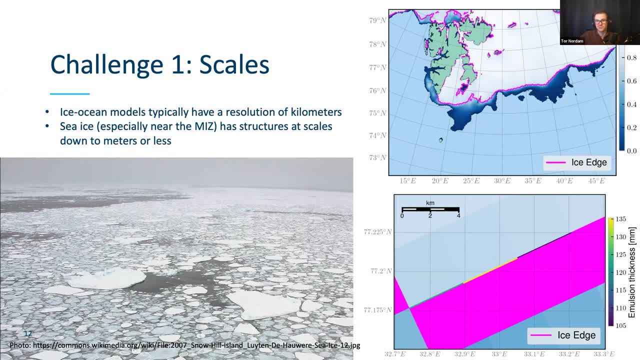 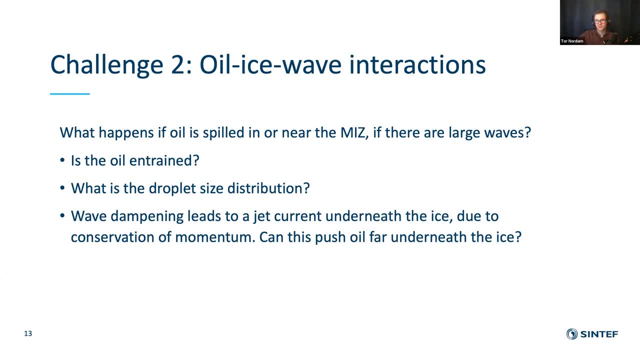 what's happening on details and small that. so this is, of course, a challenge. another challenge is that when you start looking at what's happening with ice and waves, it starts to get quite complicated, because the ice will dampen the waves, and how much and how fast depends on the thickness and the type of ice. 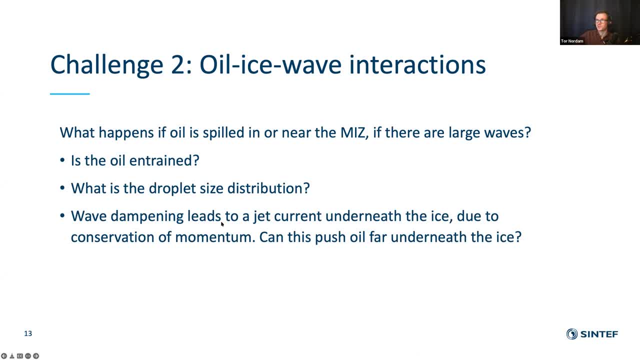 and all kinds of things, and then you can start asking questions about what happens really when you have oil in or near the marginal ozone. if you have large waves, is there going to be entrainment of the oil? what is the drawing process? so when it comes to much of that voltage, there's certain and 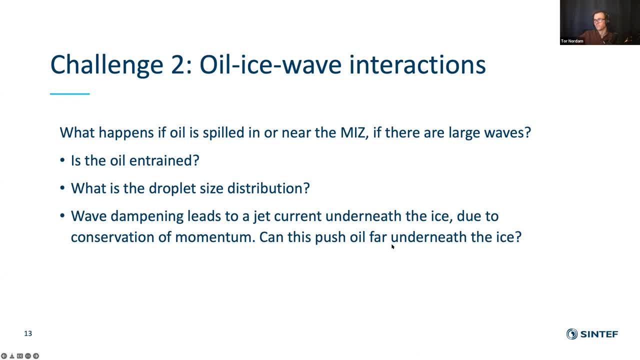 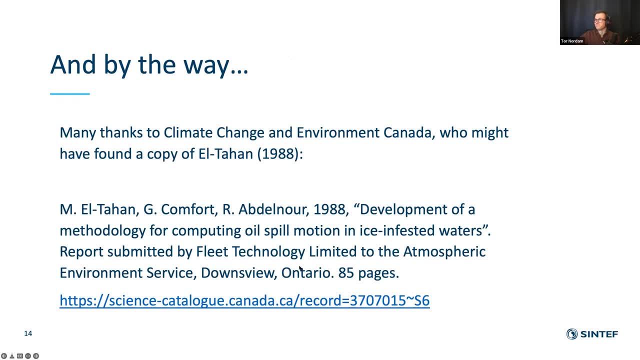 droplet size distribution going to be, and is the oil going to be pushed underneath the ice and, if so, how far? yeah, all right. um, yeah, at the end, um, this is my second to last slide. i just want to say many thanks to climate change and environment canada, who might have actually found me a copy of 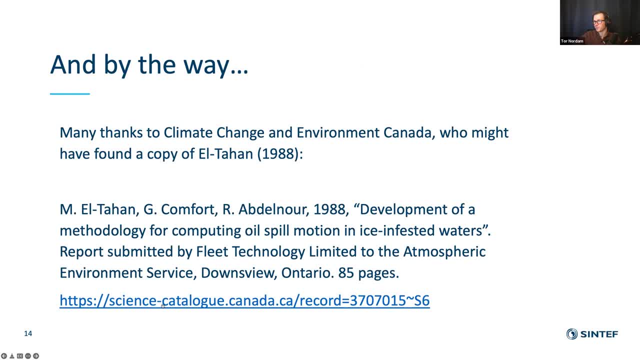 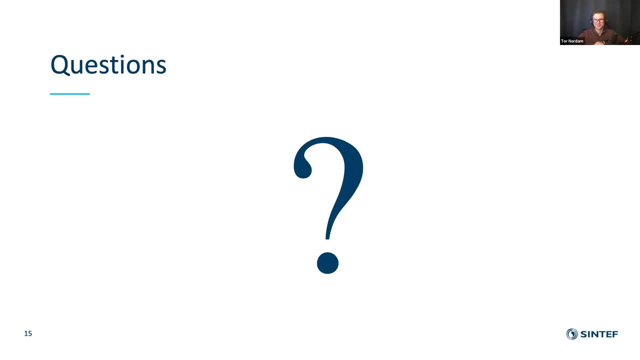 this report that i mentioned from 1988. at least they've given me a link to a catalog record in their library, so hopefully i can get somebody to scan this for me. um, yeah, so many thanks to them and uh, i guess we have 30 seconds maybe for a question, if somebody. 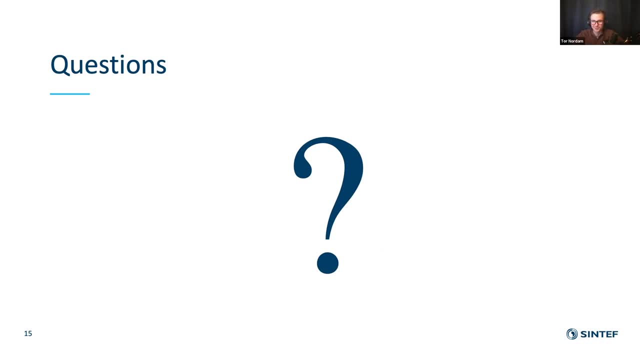 if somebody has a question. otherwise, i'm happy to answer questions later if you contact me by email or anything. yes, perfect, perfect, sir, thank you. thank you very much. this was really really nice, very interesting presentation, a very nice compliment to to amy's presentation, and i know that the all the our iarpic people have a hard deadline at the at the top of the hour. 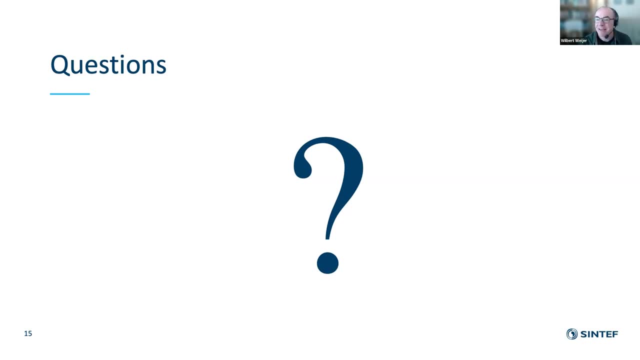 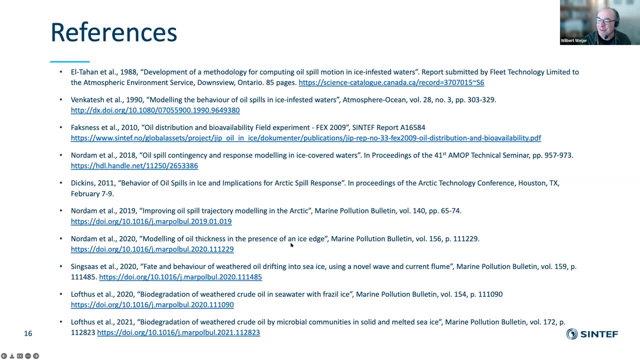 and so i do am afraid that we have to uh to cut it off here. um, so all this presentation, the, the recording of the presentation was posted on the iarpic website, and also the slides, and. um, i'm really sorry that we haven't had more time for uh, for discussion, and because this was really 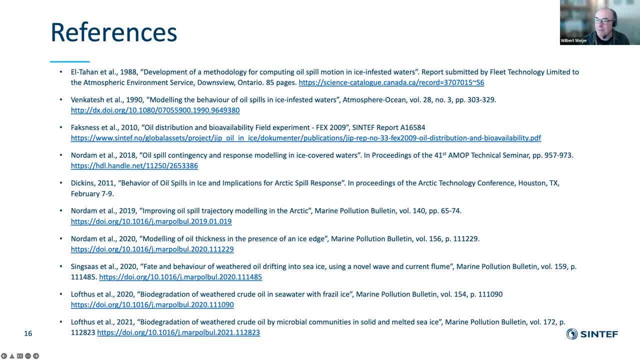 really interesting, i thought, and it was very relevant, uh, for the, for this community. i mean, i think this is really, uh, really good work. um so, with that, hazel, do you want to um close this off? um sure, i well. apologies to her for stopping the recording halfway through. 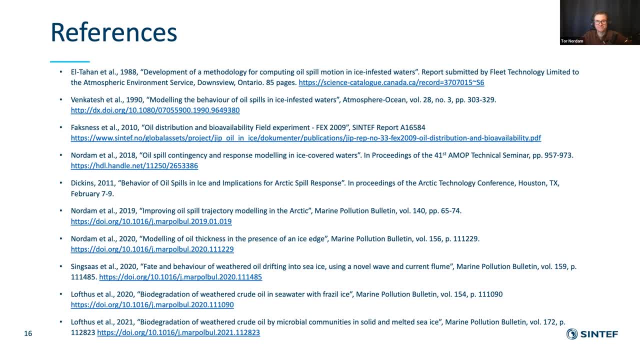 that i was trying to open the chat. um, i'm actually happy to stay on. i know that the team leaders have another meeting right after this, but i can keep the room open for five minutes if i don't know if are available or interested. yeah sure, um, so i'm happy to do that. and then i know the modeling. 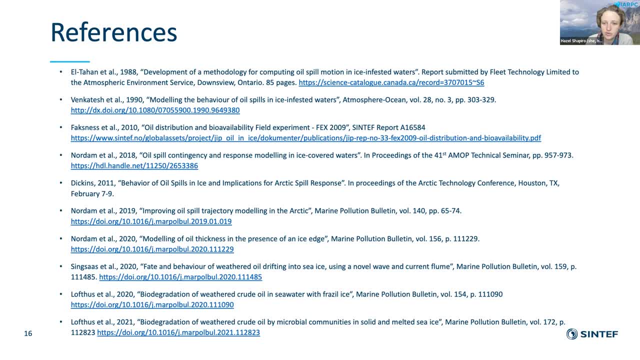 team has a related meeting coming up. i believe it's february 23rd um, and that's right. it will be on um. uh for the atmosphere, we'll be looking at atmospheric composition forecasting with the gocf model, so that that should be an interesting one, and i don't know if the post team wants to. 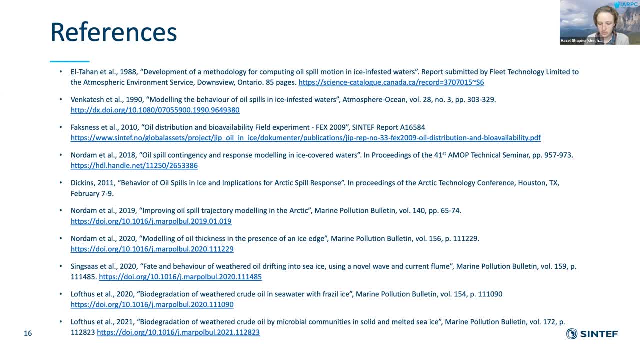 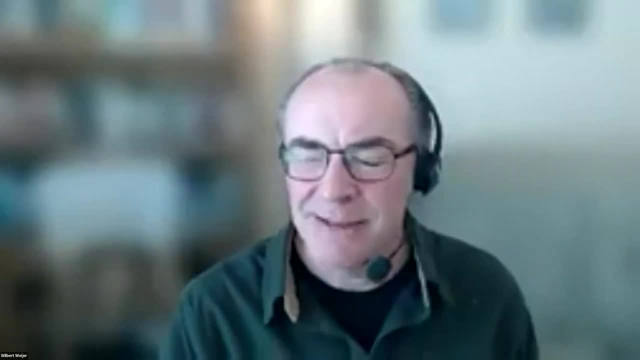 announce an upcoming meeting um and otherwise you can, you know, stay, stay tuned on the irbic website. yeah, so i'm still working on that to put together a meeting about other marine debris um work and i'm in contact with peter uh west about that. so i'm really excited about that and stay tuned for. 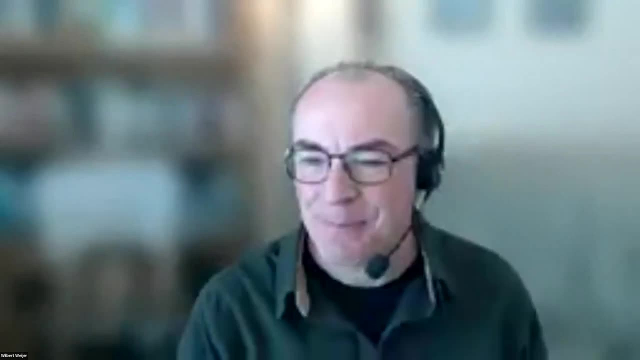 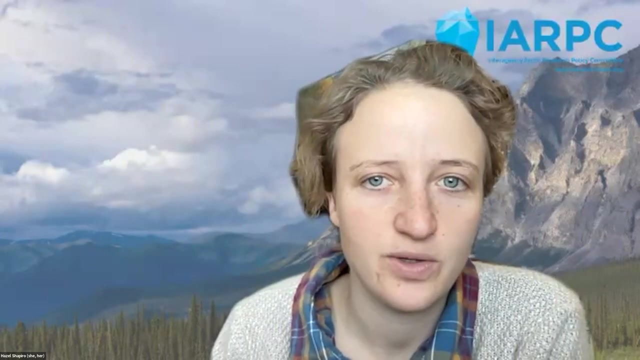 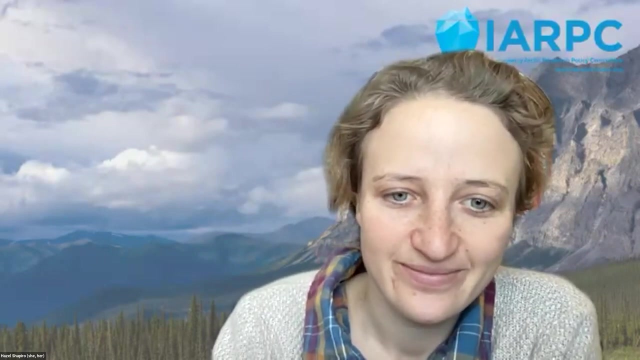 for information about that. thank you great. well, thank you all so much, and yeah again, the meeting recording will be posted shortly on the irbic website and on youtube, so um, feel free to share that around. um, will you be able to capture the chat as well, because it'd be kind of nice to have some of those questions and 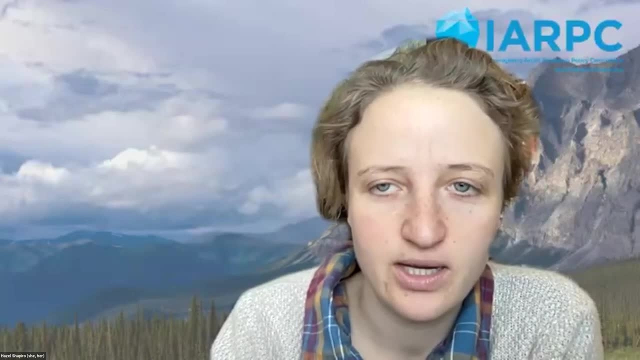 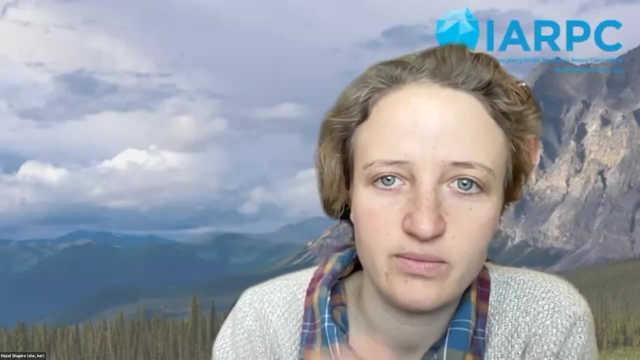 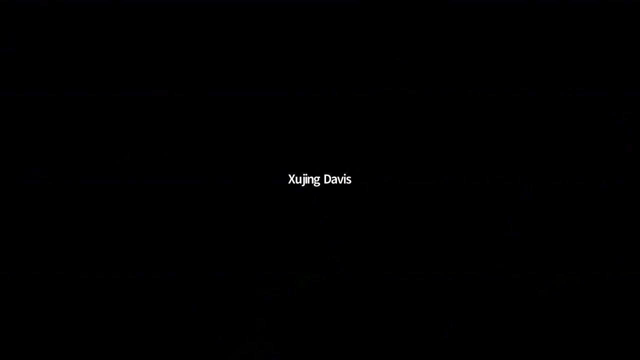 answers written. yes, i, i will capture that and put it in the meeting notes, um. and when you close out, i don't know if that happens if you're not the host, um, but often it it will save the chat on your computer. that may just be a host feature, okay, okay, see, see what. 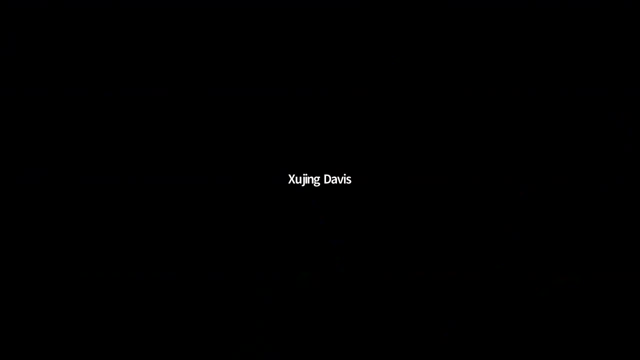 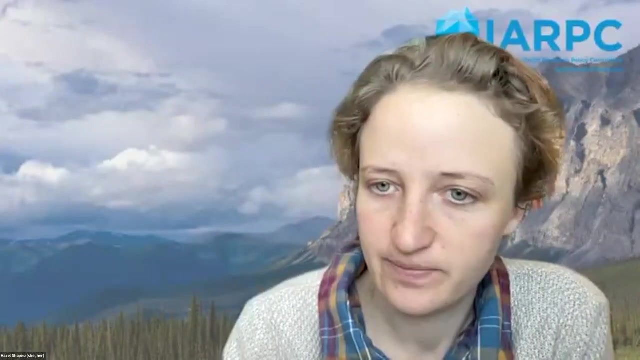 he's on. you can click at the uh chat bottom, like right hand side. that's like a three dollar dollar save chat. then you can save it. okay, yeah, perfect, so yeah, but i'll make sure all of the the chats are q a are captured in the notes. 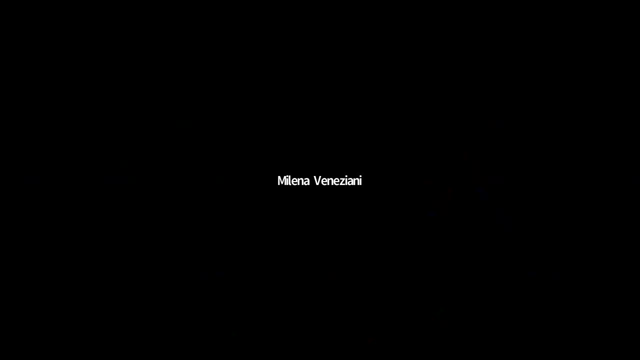 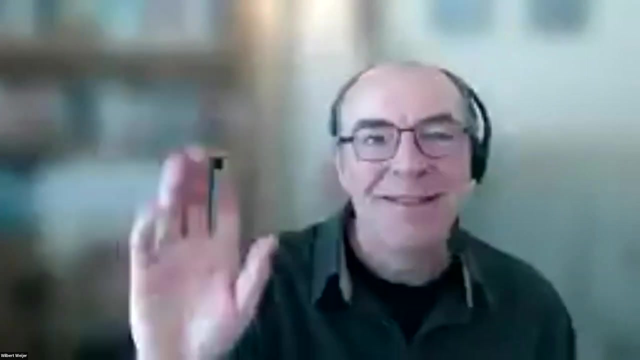 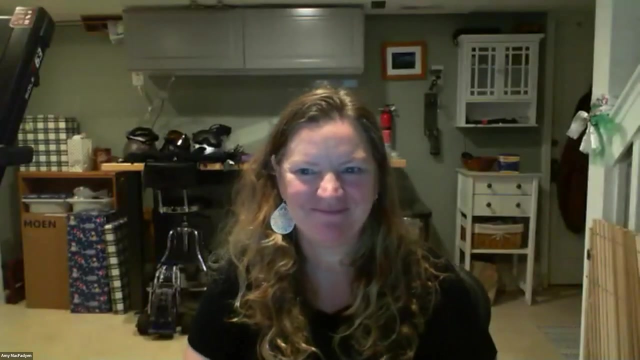 all right, great well, thank you very much. i have to uh to step off too, so thanks everybody. i really appreciate the very interesting session, thank you, thank you for inviting, thank you, thank you. yeah, thanks for the invitation.